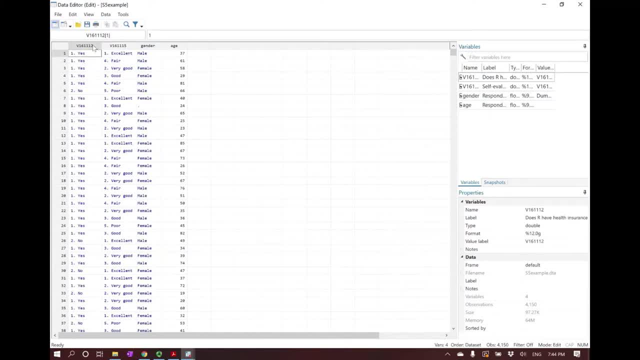 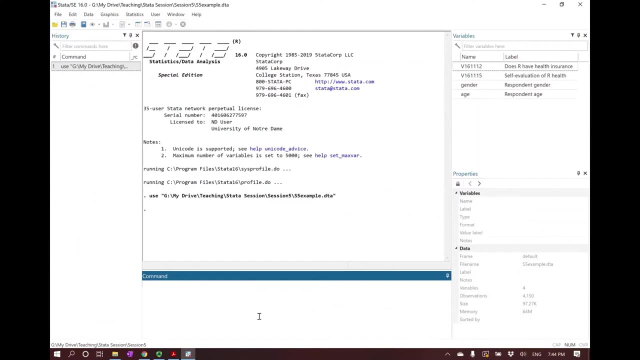 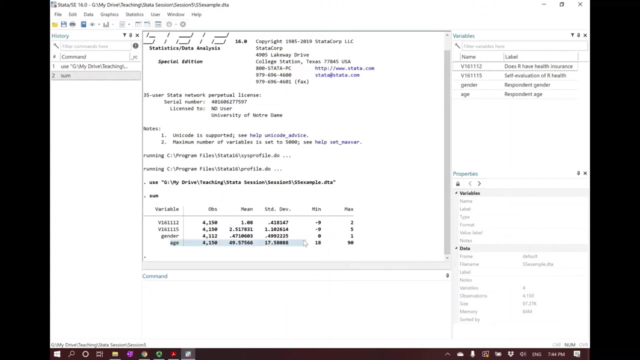 However, since the text of the three data or of the three variables are already in blue instead of red, this means that all three variables are already encoded into a numerical form. So if you do a quick summary, you can see that age is a quantitative data that takes values from 18 to 90.. 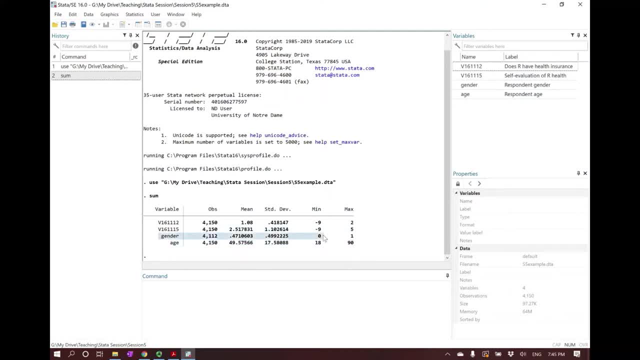 Gender is a binary variable that takes a value from 0 to 1.. Please notice that we do have some missing information for gender, The other two variables. we have some negative values here. Usually 99, negative, 99, negative, 9 are basically showing some missing response. 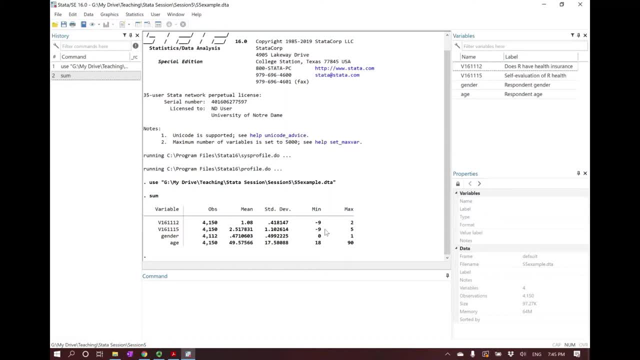 or refused response in a survey. OK, so this means actually we do need some data cleaning work to be done. OK, it looks like we are fine with the age, but in terms of the gender, we do want to look at whether female takes a value of 0 or 1. 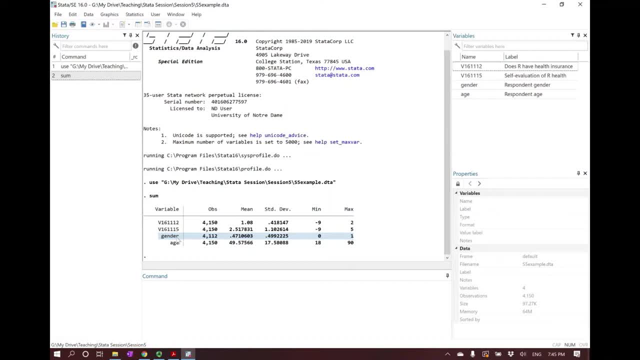 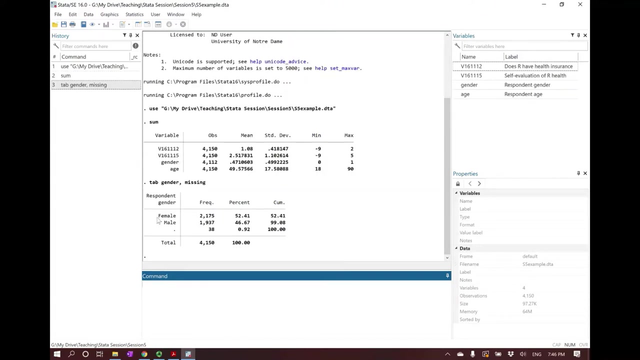 and how many observations are missing for this information. So the best way to do that is you can first tab gender to take a look at the two categories And I recommend you to include the missing observation. So if you do tab gender missing, you will see that we have one category being female. 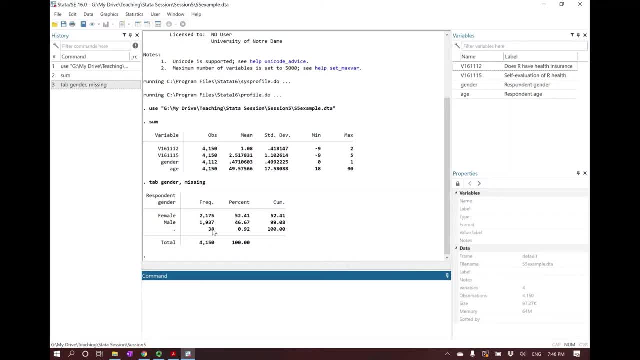 another being male, and we have 38 missing observations. In the meanwhile, if you do this tab gender again, but in this time without showing the label- so tab gender missing and also no label- you can immediately associate which values are assigned to which category. 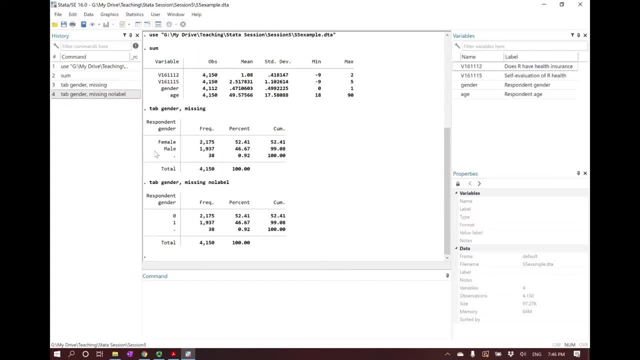 So actually the variable name is better to be called male, because in our case male is assigned to have a value of 1.. OK, but now I'm just going to drop the observations. that has them that are missing for gender. So I'm going to drop if gender is just missing nothing. 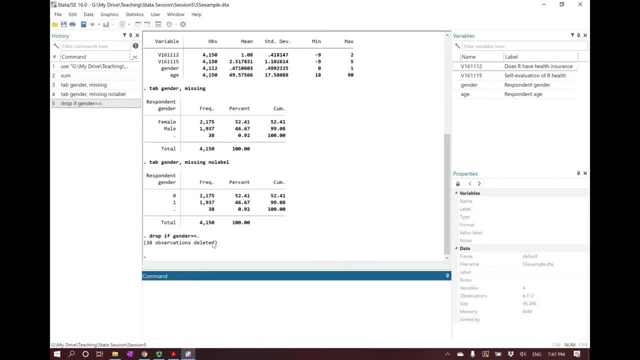 So click enter. 38 observations are deleted. OK, furthermore, I'm going to use the tab missing tab, no label to continue to study, learn and deal with the other two categorical variables. Sometimes you may also have missing data for any other quantitative variables. 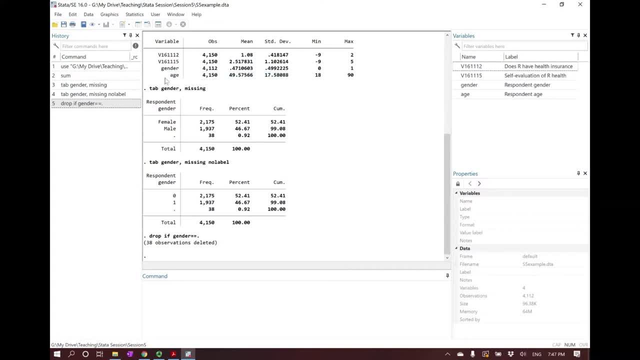 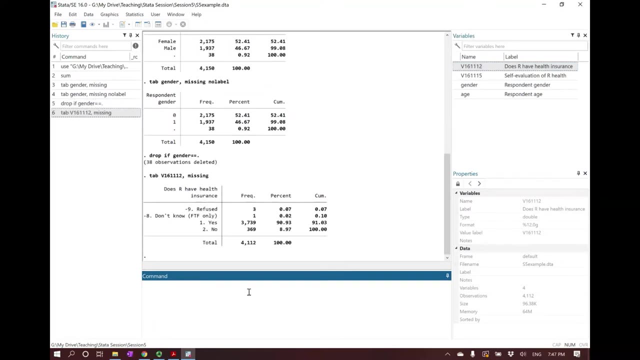 So you also want to kind of examine whether these are the case. So now I'm going to tab my first variable on having insurance or not. So tab V161112 missing. I do not have any missing categories, but I do have one categories. 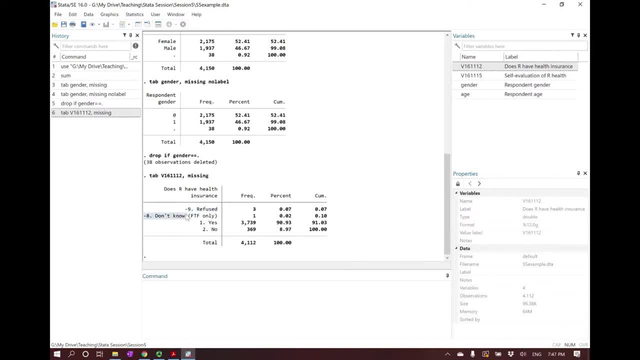 that shows refused and another category that shows don't know. So actually I have four observations. that does not give me the information on whether the respondents have an insurance, And also I'd like to know how the numerical values assigned for these four categories. 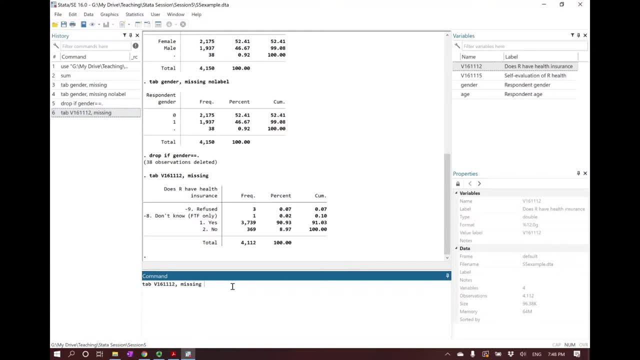 So I will do tab missing again with no label. So now I know that negative 9, negative 8 is associated with refused don't know. And I have one for yes, two for no. Now I'm going to drop if V16 equals to negative 9.. 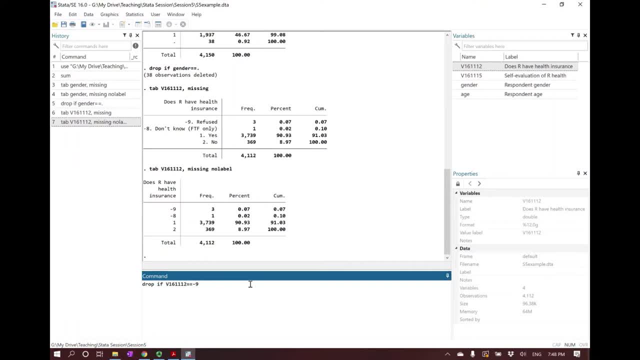 If it's a refused response I need to drop it. So three observations will be dropped. I will drop again if it's equals to negative 9.. You can do it all together. Just have like an if statement, If and war statement. 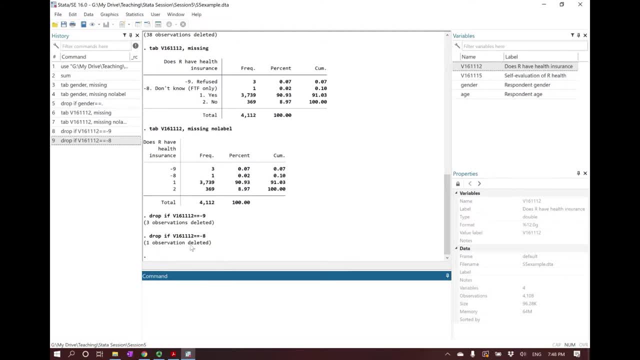 So now I'm going to enter, and one more observation is deleted. It's probably also a better idea to rename the variables. I'm going to rename this variable That's called insurance. So now I'd like to deal with the health status variable. 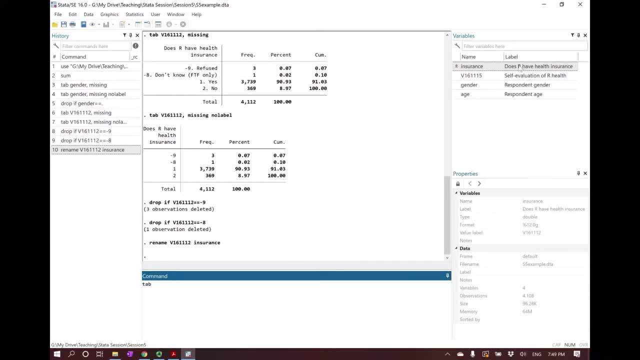 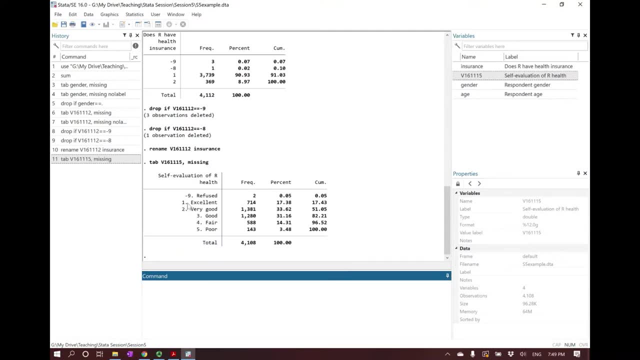 I'm going to do tab V15 missing. OK, So I have five categories And also I have two respondents who refused with the answer, So I'm actually going to. if you'd like to see the no label version, you can do that. 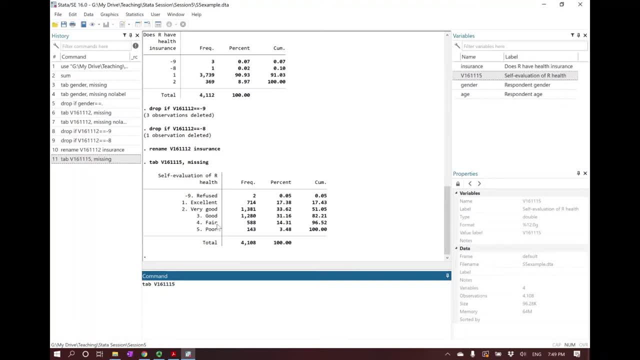 Because sometimes the name of the response, the name of the categorical text just give you excellent, very good, good, fair, poor. You don't really know what are the numerical values assigned with each category. So if that's the case, you always want to do a no label. 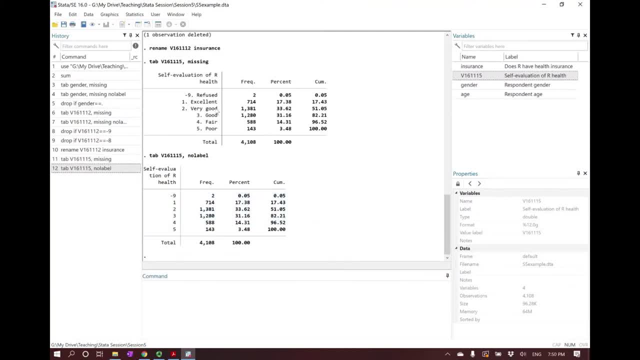 to look at the actual numerical values assigned behind each categories. So now I know that I need to drop the negative 9.. If this value equals to negative 9.. Remember, after the if statement we want the double equal sign Because we are kind of testing for that equality. 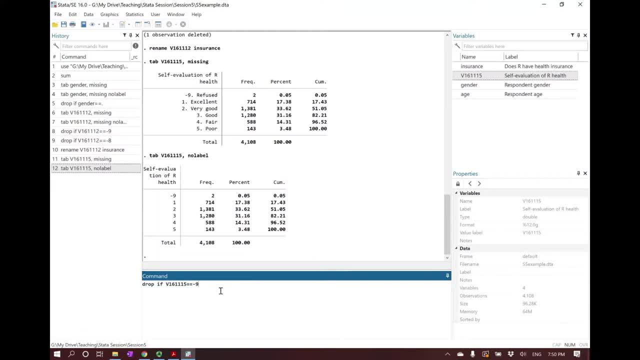 If this equality is valid, we're going to drop. We're not defining some information, So if I drop, I will have two observations deleted And I'd like to name this variable Rename to be, for example, health. OK. 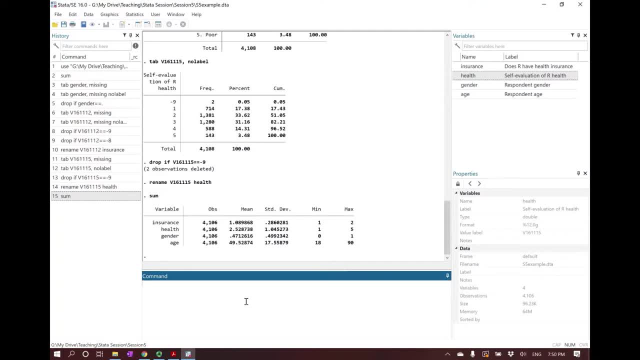 So now, if I sum all my variables again, I have some well-cleaned data set where I have 4,106 respondents or observations left And insurance from 0 is 1 to insurance from 1 to 2. So it's a binary variable. 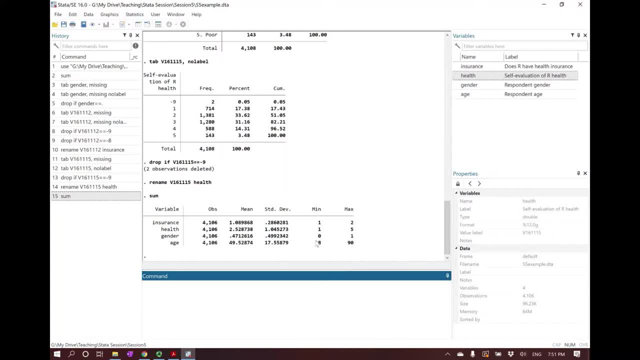 Health is from 1 to 5.. Gender is 0 to 1.. Age is from 18 to 90.. Of course you can. if you'd like to have insurance 1 being yes and 0 being no, you can just quickly use the recode. 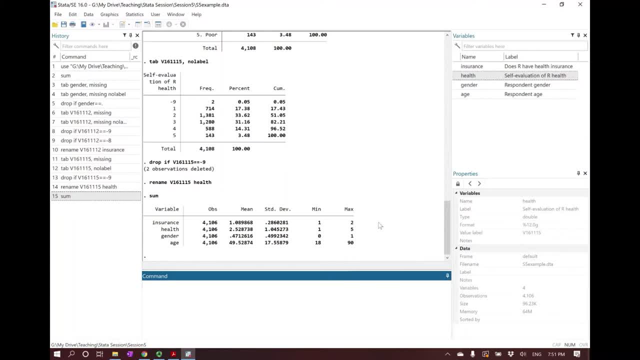 And just recode insurance. 2 equals to 0.. So it's going to be recode insurance. If you want to do 1 is 1, that's fine, Because 1 is still going to be 1.. But 2 is going to be 0. 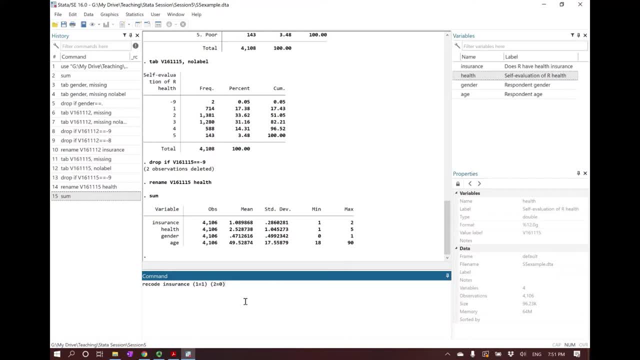 OK, If you'd like to do that, that's fine, But I'm not going to do that because these are just categorical variables. I'll just leave it for the categorical variables in this case. Sometimes I do want kind of more binary variables where the values are either 0 or 1.. 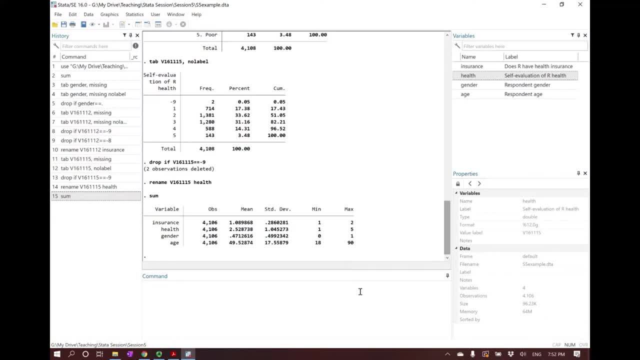 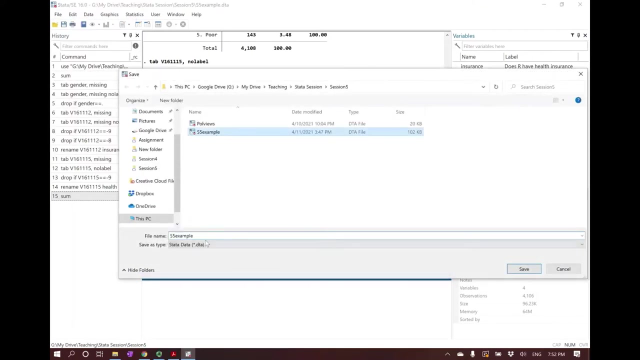 If that's the case, I would like to recode. OK, So this is the more cleaned version, where I dealt with many of the things with my variable And I also dropped many observations compared with the previous raw data. So it's actually always a good idea to just save another version. 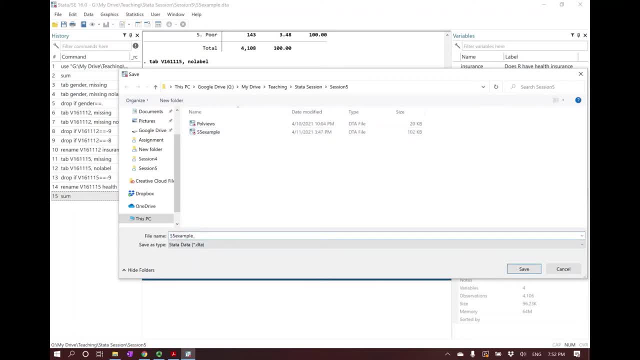 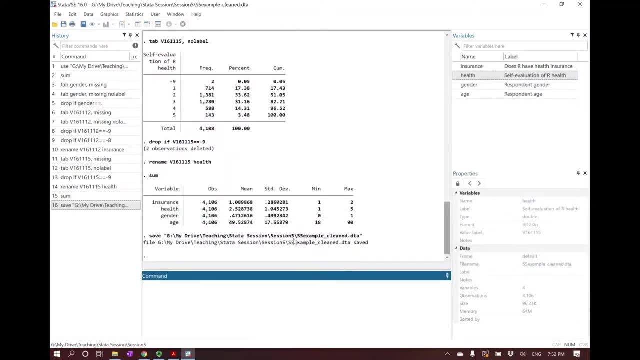 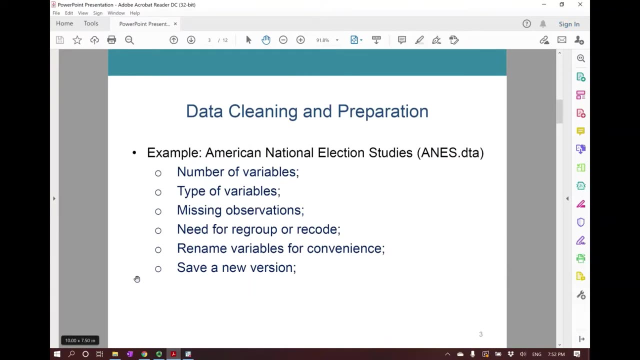 For example, I'm going to save it as session 5 example- cleaned. OK, You still have a version for your raw data and another version for your cleaned data, OK, So to just summarize what I did, sometimes whenever we load a new data set, 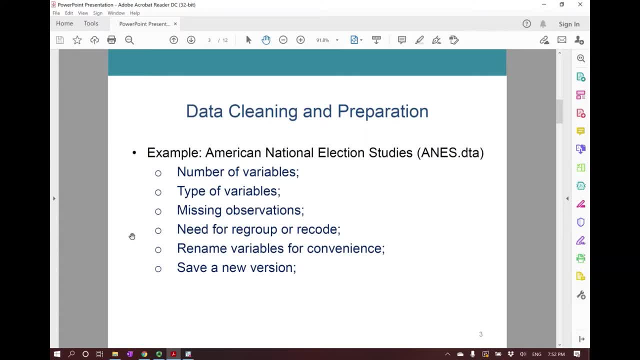 it's always better to do some cleaning and preparation And definitely always get familiar with the variables and the data that you are working with. You want to look at how many variables you're working with, type of variables and also, if there's any missing observations, how you want to deal with the missing observations. 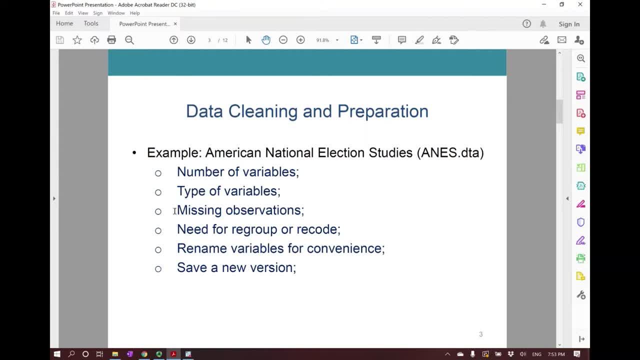 Sometimes, if it's not a primary variable you're going to examine and it has a lot of missing information, instead of dropping those informations, you may consider not using that variable at all. So sometimes it's something to consider. Furthermore, you want to look at whether there's need to regroup or recode. 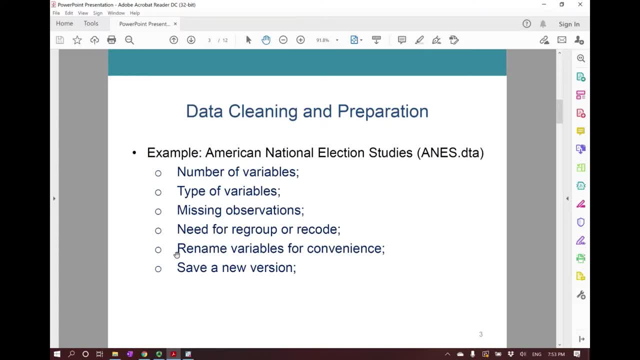 some of your values? OK. You want to rename the variables for the convenience, and you want to save a new version? OK. So in the next I'm going to talk about the Stata comment for constructing a confidence interval. The comment is actually very simple. 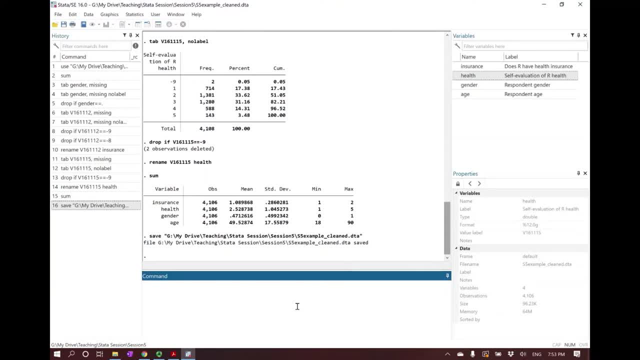 But if you recall the concept of confidence interval from the class, we're going to construct a confidence interval for age. This is the only quantitative data we have. So if I am going to do a sum, suppose that we're trying to look at the information. 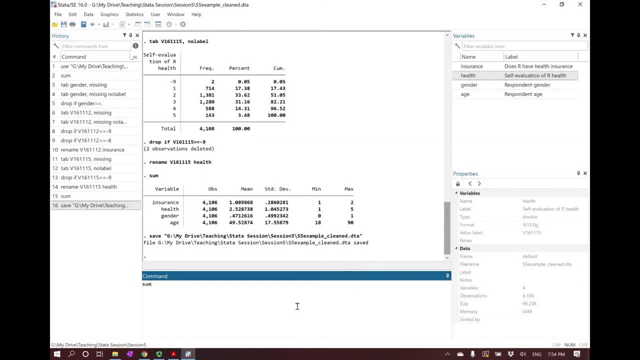 or understanding gender, age and health and insurance purchasing behavior for everyone in the US, then we collect a sample of around 4,000 respondents. right, Because in statistical inference we need to care whether we're winning or losing. We need to care whether we're working with population or whether we're working with a sample. 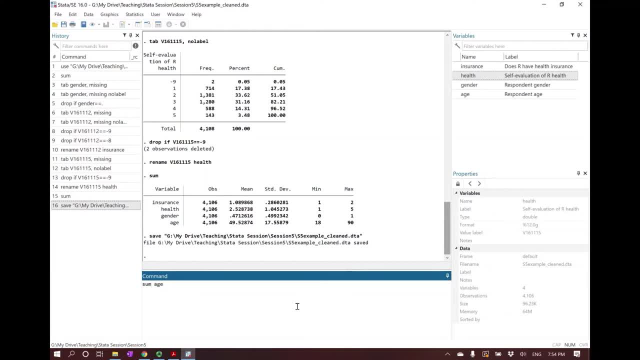 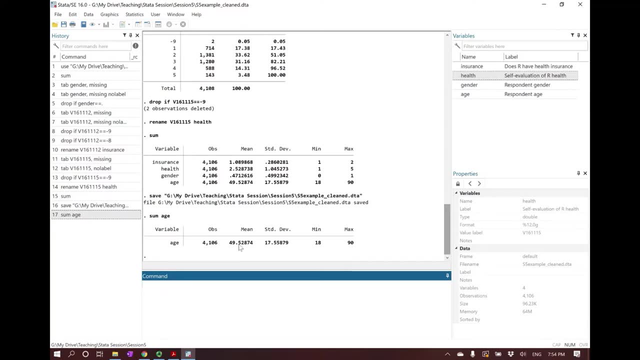 So now we have a sample. So if I'm going to sum age, my sample mean, my sample size is 4106.. My sample mean is 49 something And my sample standard deviation is 17.55.. OK, So using the traditional way to manually calculate a confidence interval, 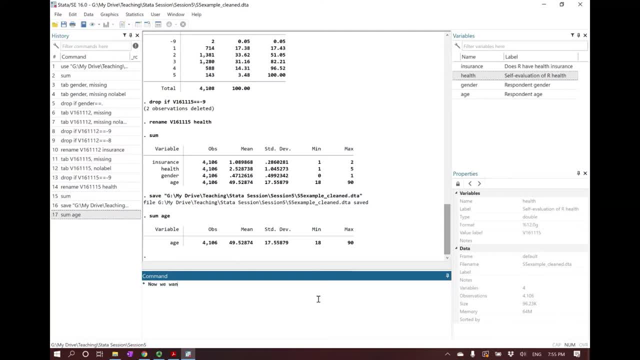 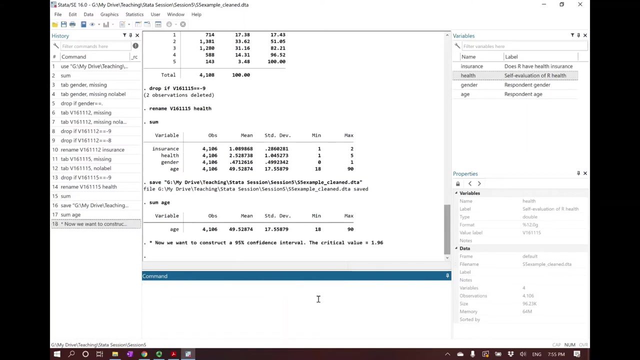 basically now we want to say construct a 95% confidence interval. If you recall, the critical value is 1.96, right? So I'm actually going to use Stata as a calculator to calculate the two bounds of my interval. So the lower bound would be the sample mean, which is X bar. 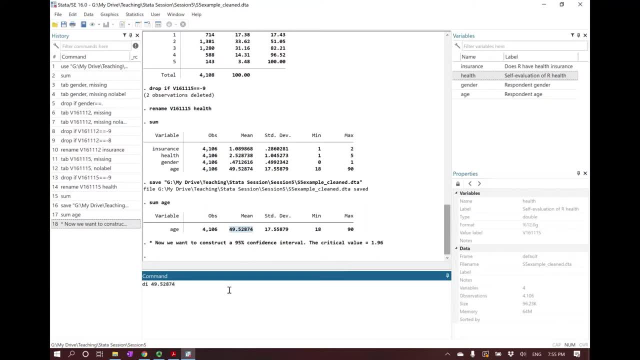 I'm going to copy this number. Copy and paste: Minus 1.96 multiplied by the S and divided by the square root of N, So that's going to be 4106.. OK, So I'm going to click Enter. 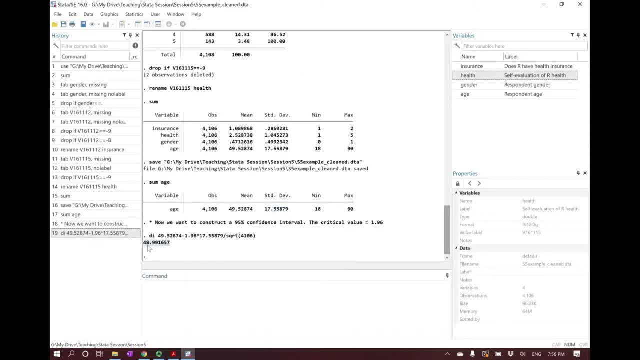 And it calculated that the lower bound of the interval is 48.99.. Now I'm going to calculate the upper bound, which I just need to change the minus sign into a plus sign. I'm calculating X bar plus 1.96 multiplied by S, divided by the square root of N. 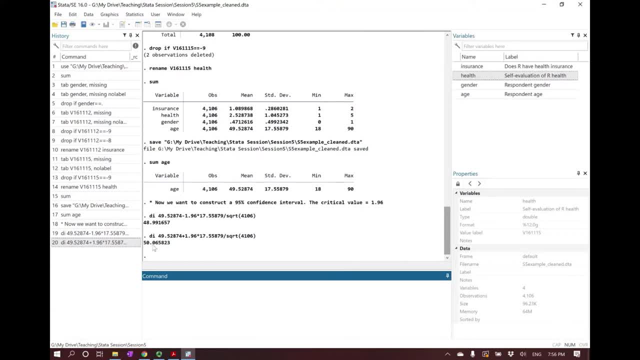 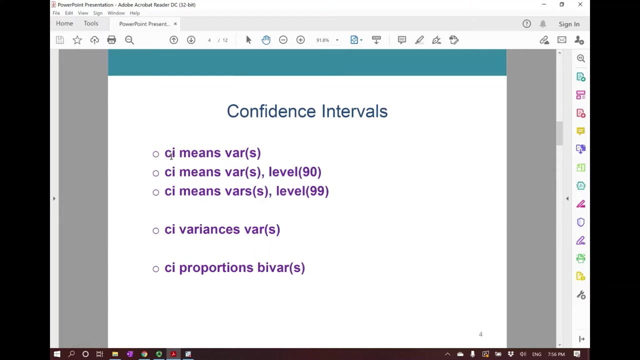 Click Enter is 50.066.. OK, This is how we did in our regular lectures. But if we know the sample and we know the sample information, we can actually use a one-line comment to calculate this interval, And the comment is called CI stands for confidence interval. 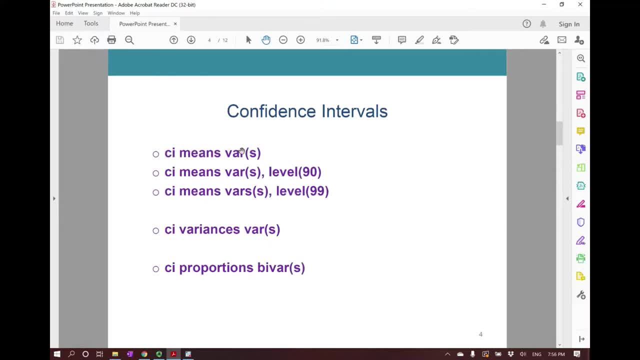 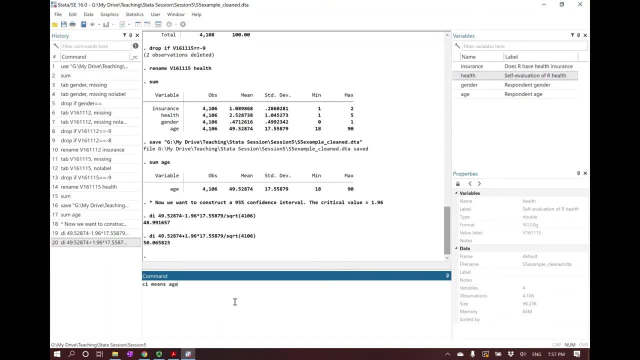 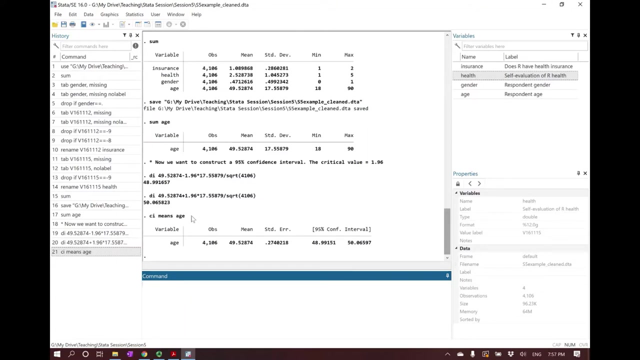 CI means and the variable. You can calculate the confidence interval for a list of variables at the same time, OK, So that's why I have a plural here. Let's calculate CI means, age. That's it. If you click Enter, by default Stata will always choose an alpha of 5%. 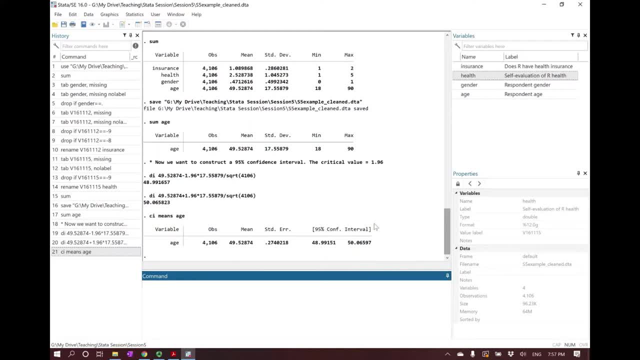 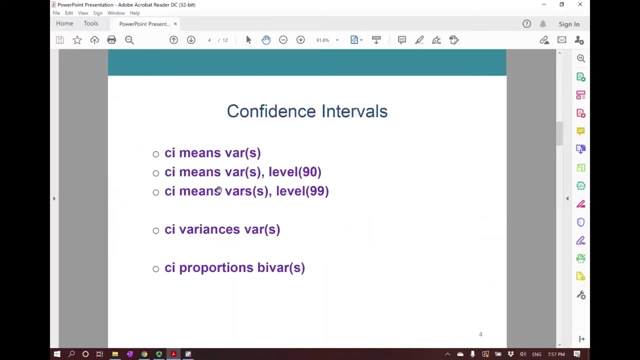 or always choose 95% confidence interval. But, as you see, we calculated correctly: The lower bound was 48.99.. The upper bound is 50.066.. OK, So we do have some other options, For example, if you'd like to construct the 90% confidence interval. 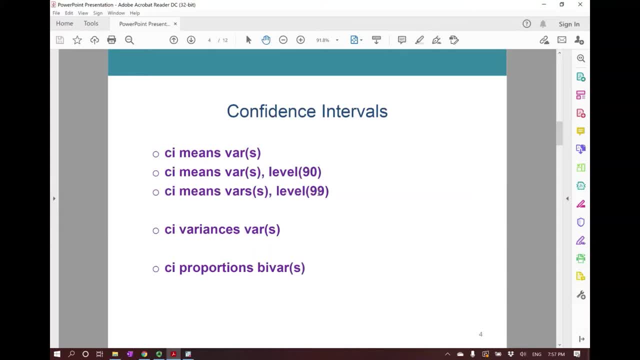 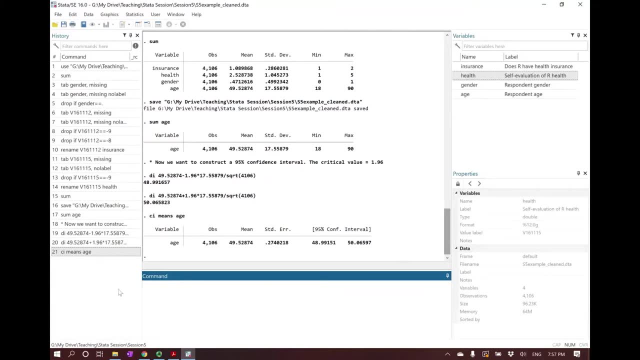 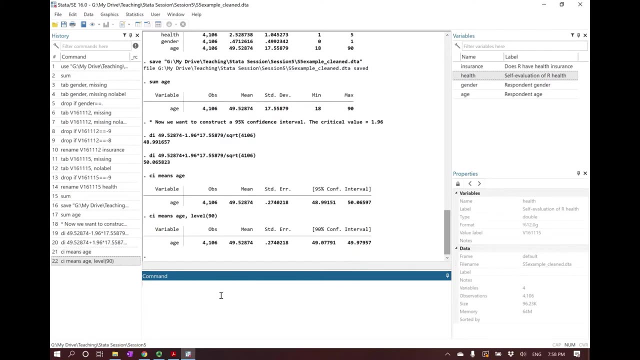 or the 99% confidence interval. you just need to give an option and override is 95% default. So the way you do that is just: CI means age Level 90. So you got the 90% confidence interval. If you calculate, CI means age 99,. 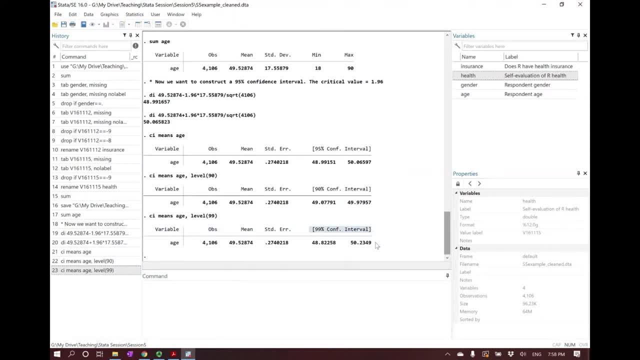 you got the 99% confidence interval OK. So these are just very easy ways to calculate confidence interval. If we're going to supposedly treat all of the variables as quantitative variables, you can calculate a list of variables At the same time. 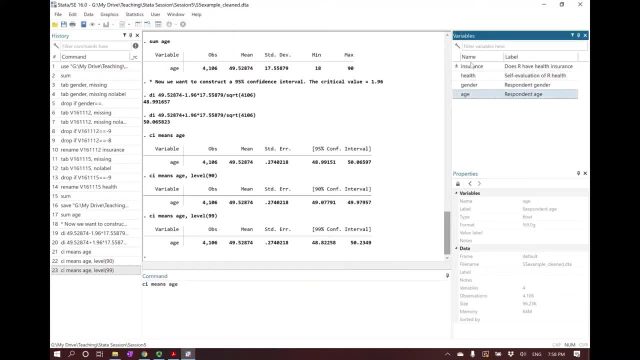 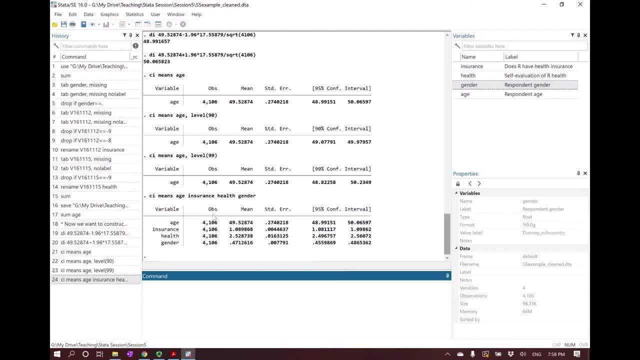 So I'm going to do say age insurance, health and gender. If I click OK, you can calculate. It will still give you the information on the mean and standard error. If you see, here standard error is a little bit different than the standard deviation from the sum. 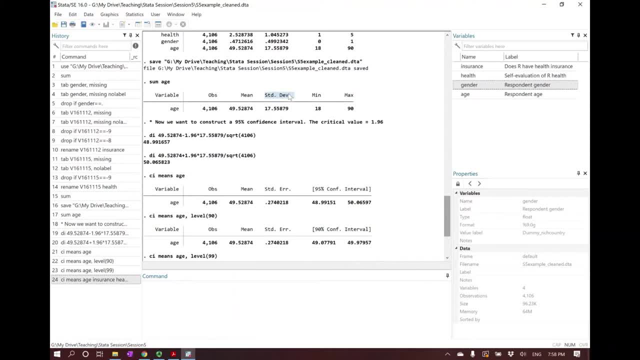 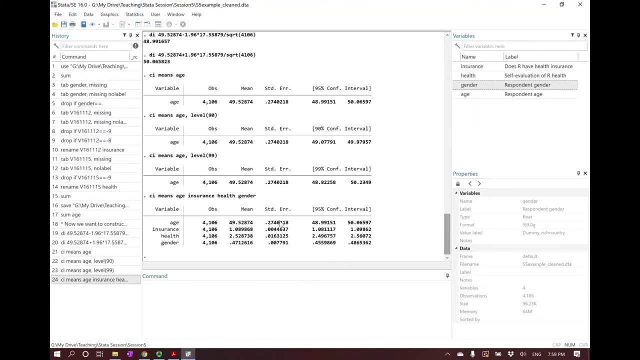 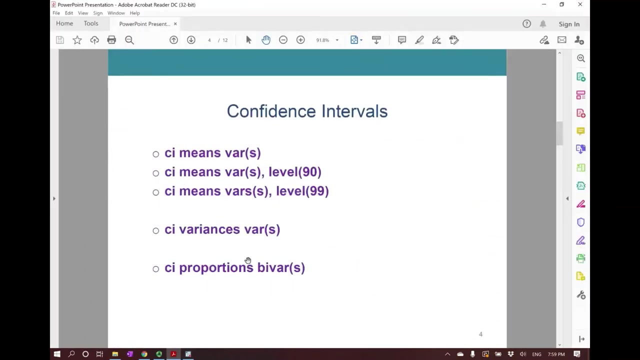 Standard error is the standard deviation divided by the square root of n. OK, So that's basically mean plus and minus. That's standard error. that gives you the interval, So you could calculate a list of variables at the same time, OK. On the other hand, if our target parameter is, for example, population variance or population proportions, 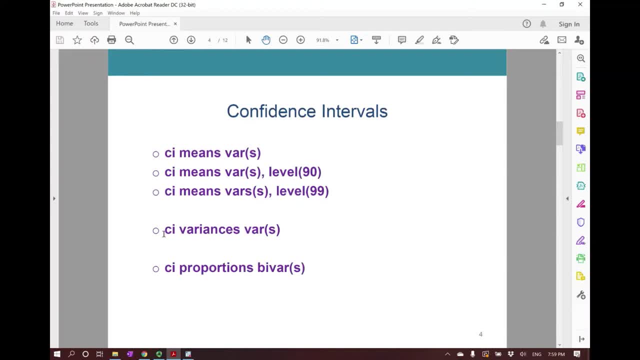 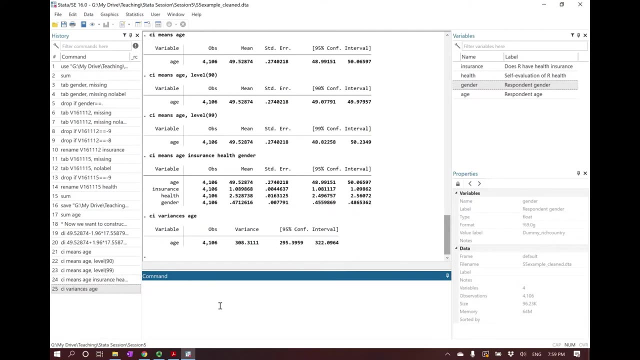 you could also use the same CI column And to calculate, for example, the 95% confidence inference for a population variance. So, for example, if I can calculate CI variance, age, So now I calculated a different 95% confidence interval. 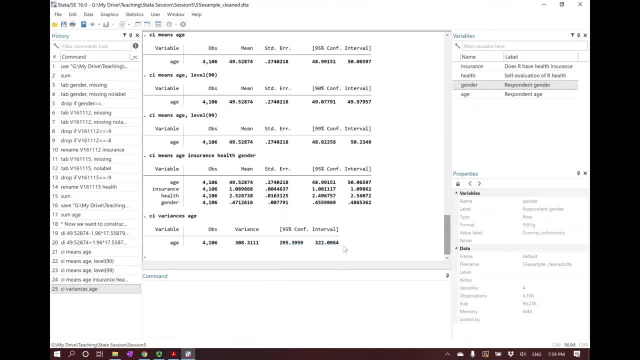 This is based on that. the sample variance is my sample statistics here And I constructed a 95% confidence interval around my sample variance and hoping that my population variance is enclosed within this interval. OK, So same thing for population proportion, And whenever we are calculating a population proportion, this is usually good for qualitative data. 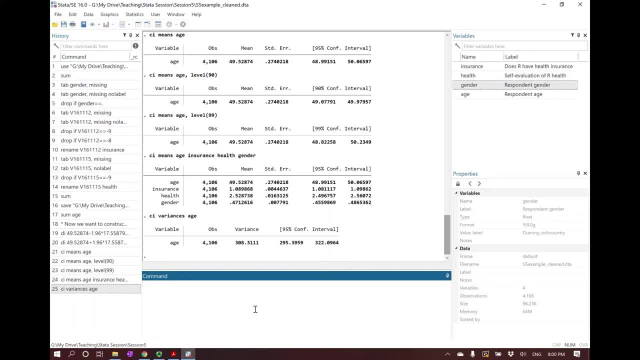 We want to. we do not have a mean or a variance or a standard deviation. Instead, we want to look at the percent of one category or a percent of one group among the population, For example, if our we want to know if the population proportion for female gender is actually a binary variable. 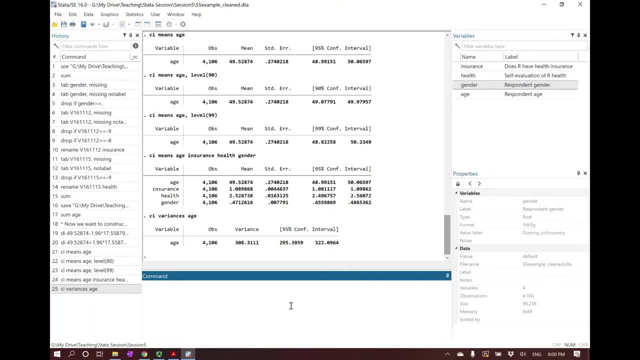 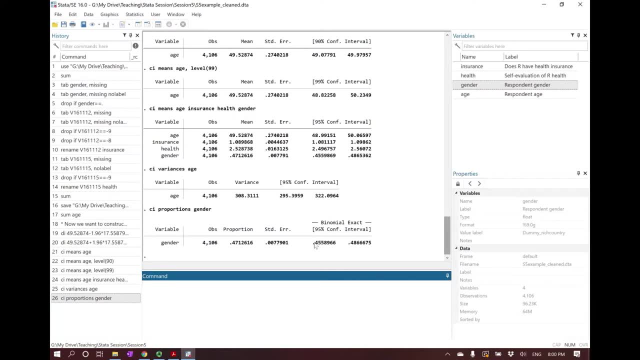 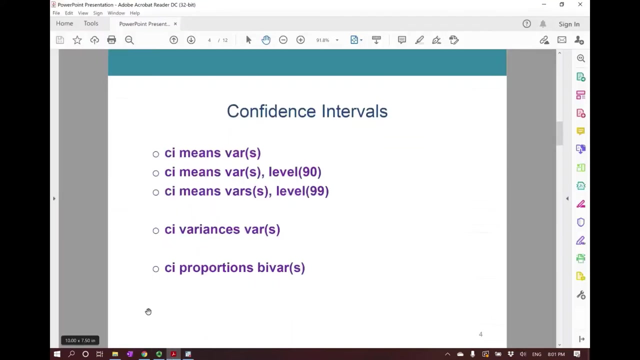 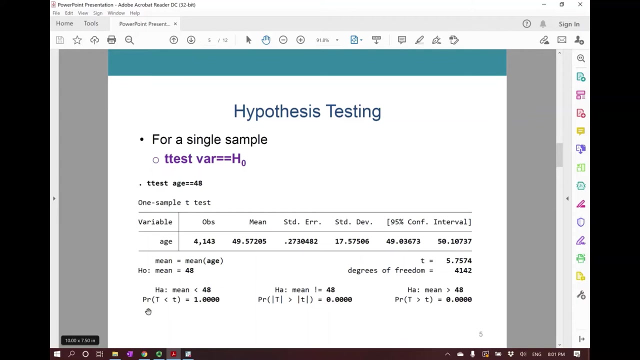 is a categorical variable So you could actually calculate CI proportions, gender. It will calculate a confidence, 95% confidence interval for that population proportion which is the percent of male in the US. So this is the confidence intervals. The next one we're going to talk about is the hypothesis testing. 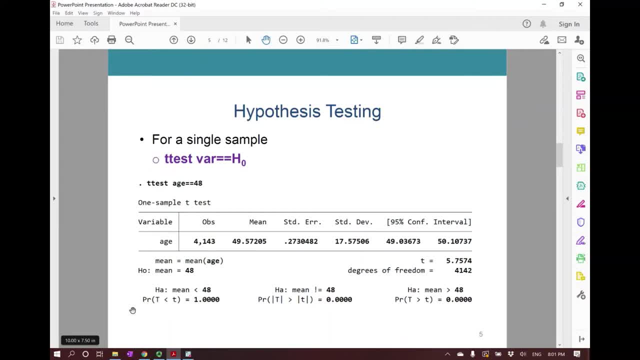 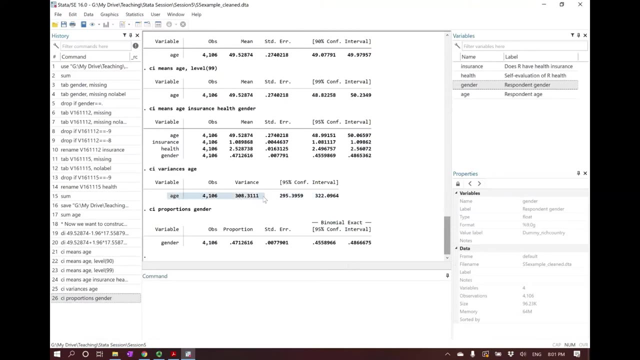 All the comments today are very simple. It's just a matter of fact Being able to read this data output OK. So suppose now we would like to test whether the age so, for example, the average age or the mean age of the whole US individuals. 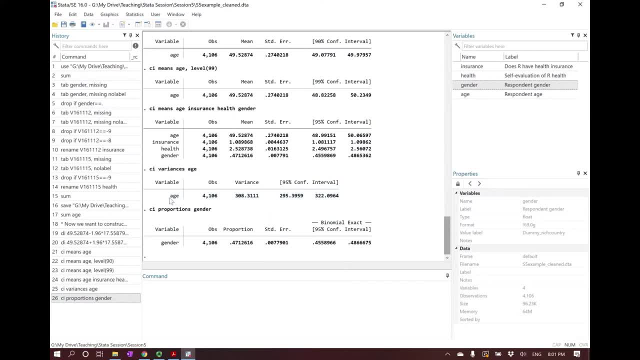 the average are, say, above 48.. Right, So now we want to test if the true mean age, the true mean age, is above 48. So actually, my null hypothesis is going to be: mu equals to 48. And my alternative hypothesis is going to be mu greater than 48.. 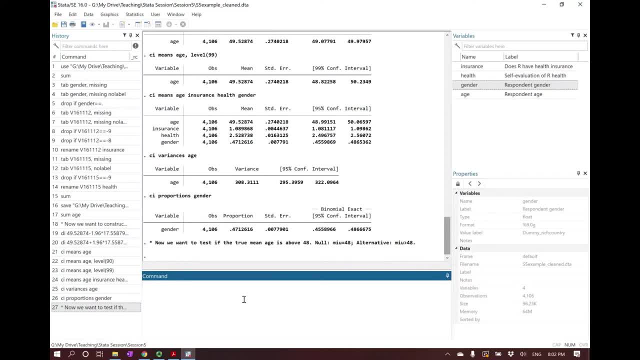 OK. However, if you're using this data for hypothesis testing, we don't really need to care about whether we're doing an upper-tailed test, a two-tailed test or a lower-tailed test. The comment is exactly the same. 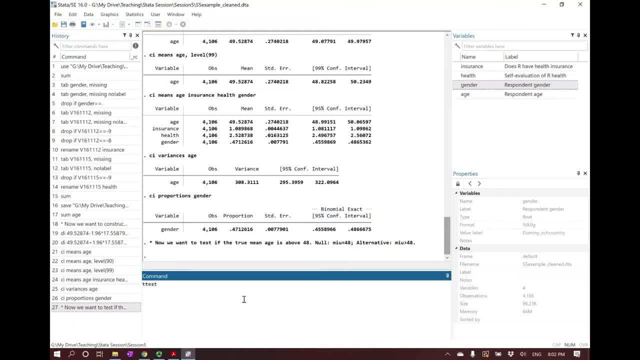 Basically you just need to do t test. age equals to 48.. 48 is the claimed value under H naught. So you always just test whether age is, say, 48 to see whether Stata can reject that null hypothesis. Stata will always do the three tests altogether. after these comments. 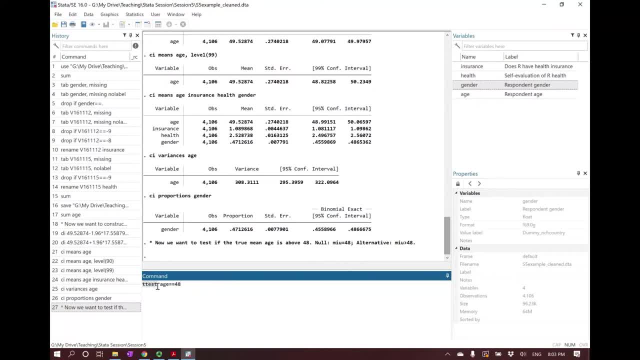 OK, And we are always. the code is always going to be a t test, even though for a large sample we always said that it's going to be a z statistic using a critical value from the z table. But Stata will accommodate that for either large sample or small sample. 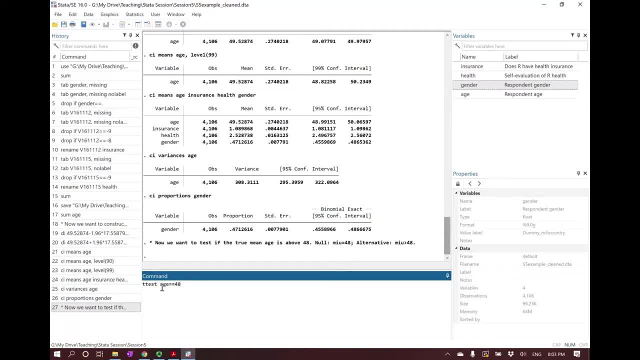 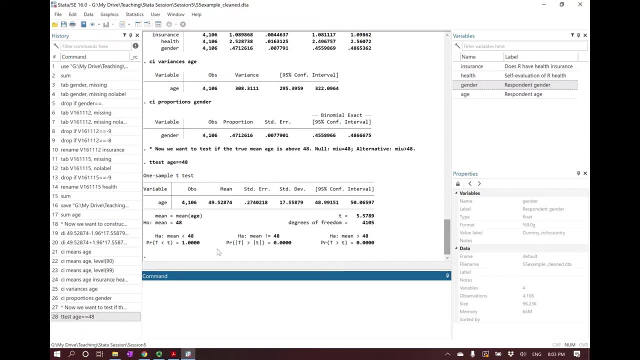 Because the t statistic will converge to z for a large sample, So the comment is always called t test. So if you click enter, we're going to take a look at the result. OK, So first of all, Stata will still. 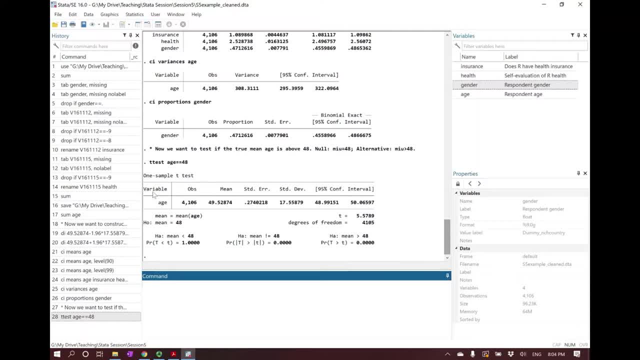 even though you're performing hypothesis testing, Stata will still report several important summary statistics for you, including the 95% confidence interval. So it gives you the observation, the sample mean, the sample standard deviation, which is this one, and the sample standard error. 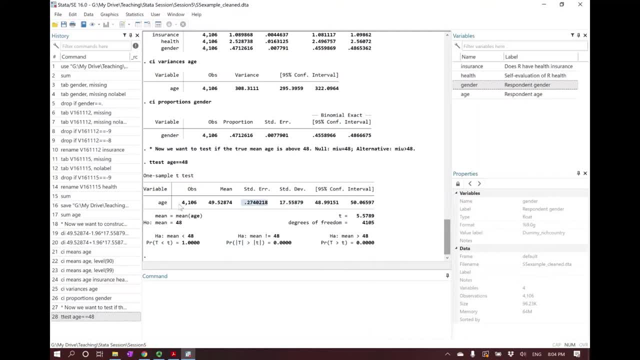 which is the sample standard deviation divided by the square root of n, And it will give you the 95% confidence interval. At the same time, Stata will show what is your non-hypothesis, And no matter what type of test you want, 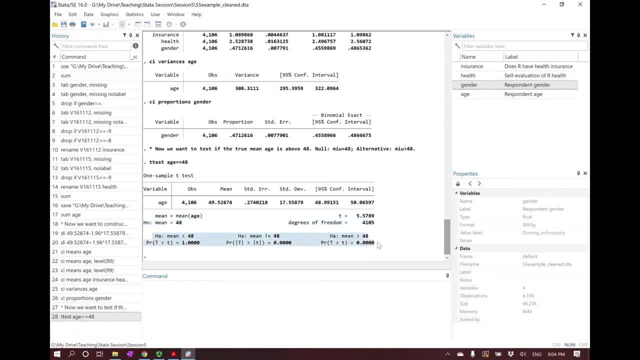 Stata will report all three tests for you. It will always do a two-tailed test listed in the middle. So the alternative hypothesis is that this mean age is not equal to 48.. OK, And it will also give you the alternative where the mean is less lower-tailed test. 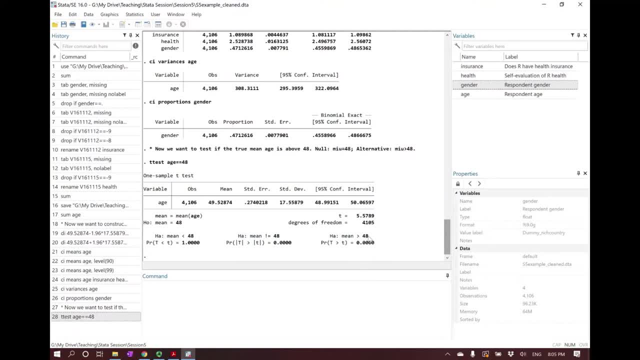 and then when the mean is lower, the mean is higher- the upper-tailed test. So you don't really need to worry on specifying your alternative hypothesis in the Stata comment. OK, So let's try to recall our traditional critical value method. 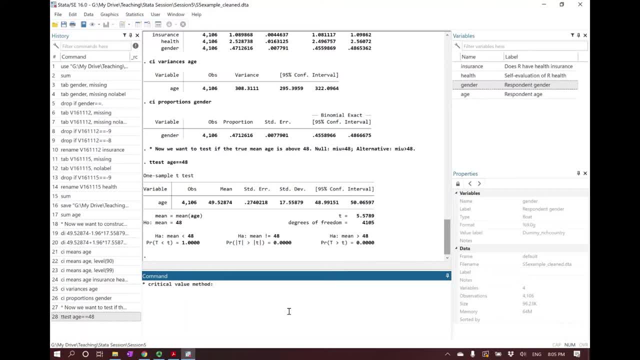 where, for example, if we want to do- let's probably do- a two-tailed test, because the critical value was just one point, One, point nine six, which we just used before, And the t statistic is something we need to calculate. 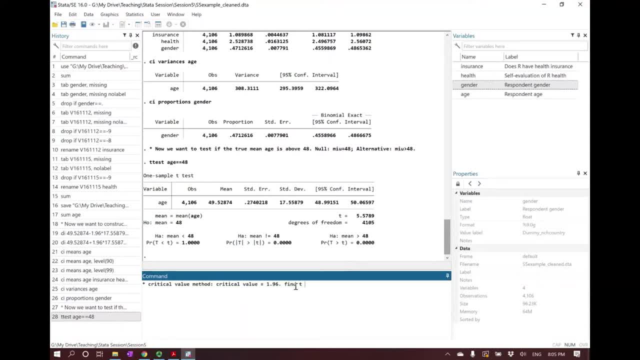 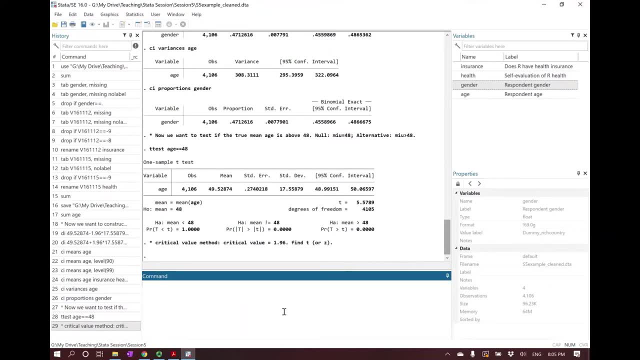 So we need to find t or z for a larger sample. So let's quickly use Stata as a calculator to see if we find the correct test statistic. So display: I have to have x bar which is forty-eight, So x bar, forty-eight minus mu zero. 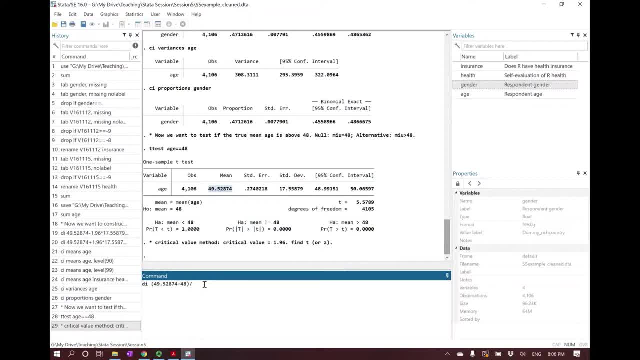 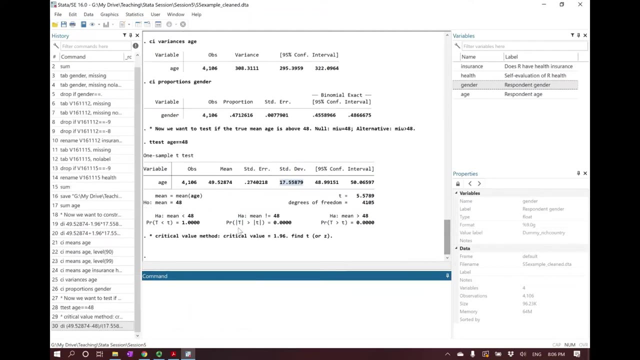 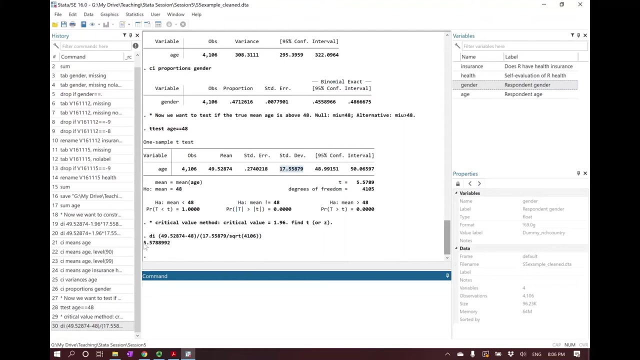 which is the value under H naught, divided by the standard deviation, divided by the square root of n. Four, one oh six. Now I'm going to click enter. I have a z statistic or t- Stata does not distinguish here. That is five point five, seven, eight, nine. 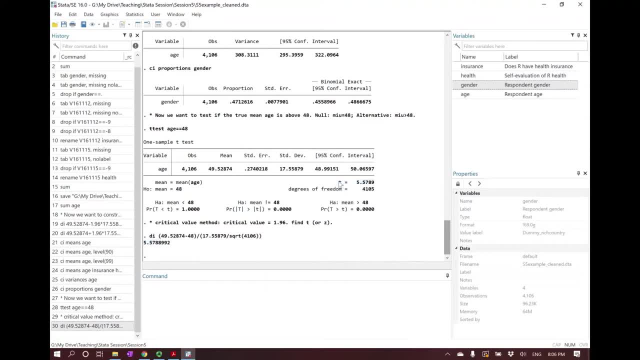 which is always reported here. OK, And it also reports the degree of freedom. However, it will still already converge to z statistic. OK, According to the traditional method, since t statistic is greater, equals to five point five, eight greater than one point nine six. 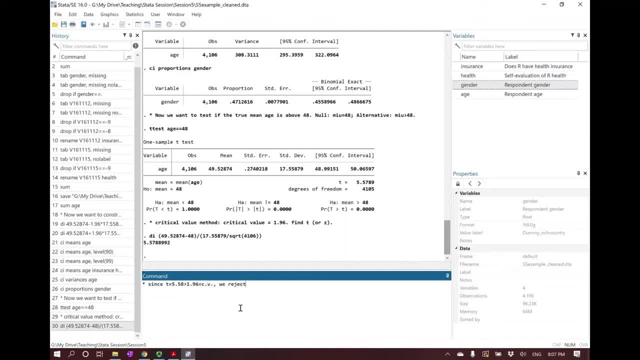 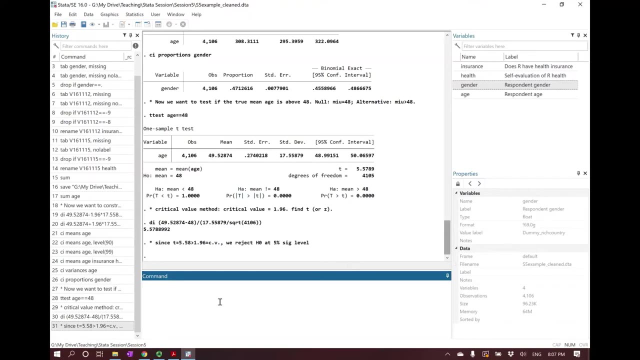 being the critical value, we reject. H naught at five percent significant level. OK, Remember this is what we did in the regular lecture. However, in empirical research, and especially in Stata, the most way we look at is through the p-value method. 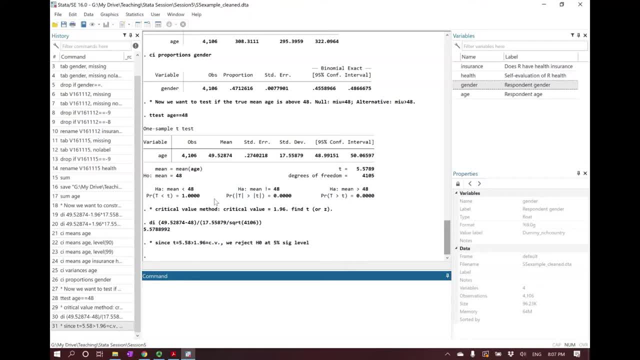 because we do not have to specify a significance level. So therefore, using the p-value method, you could just say: since the p-value is equals to point, zero, zero, zero, zero, so we can reject H naught at one percent, five percent. 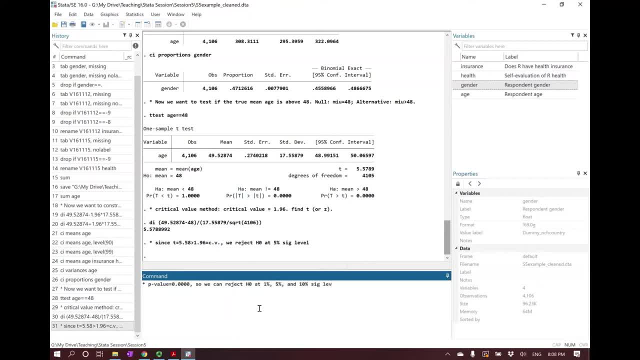 and ten percent significant level, Right? So in a non-technical way of interpreting this, is that the true mean age for US residents, suppose, is different from forty-eight. If it's a one-tail test, we'll say it's greater than forty-eight. 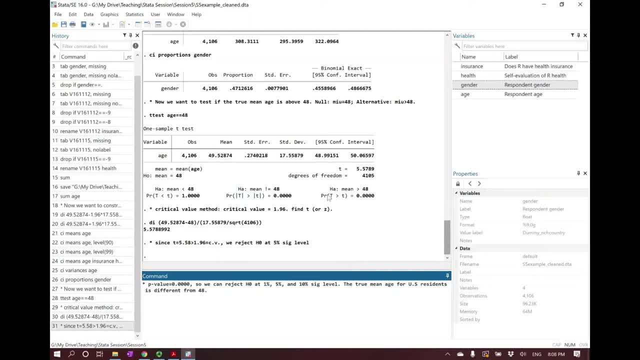 For the one-tailed test we can also reject at the one percent, five percent and ten percent level. So if your research claim is about a one-tailed test, you can say that the true mean age for US residents is greater than forty-eight. 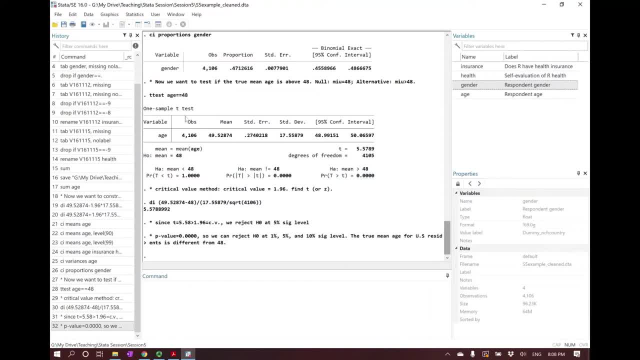 OK, So this is just the one line comments for a hypothesis testing for one single sample. Again, it will create this ninety-five percent confidence interval for you, So sometimes we do not even need to use the CI means comment. You could directly always use. 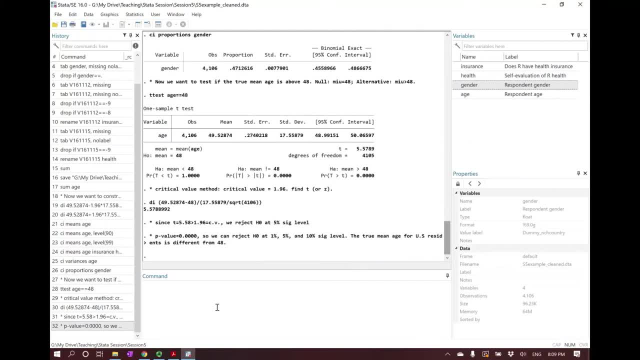 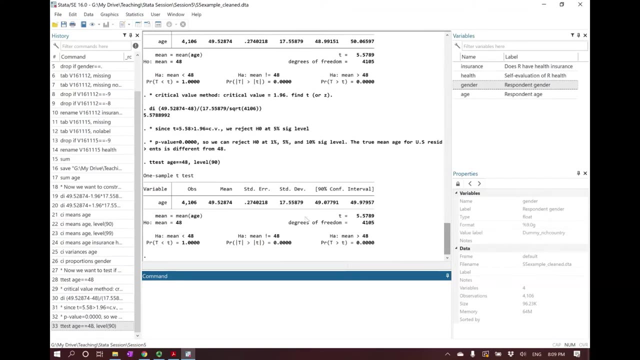 the T test and it has everything for you. OK, Of course, if you do the T test, H equals to forty-eight, with a comma showing a level of ninety percent. OK, So your hypothesis testing will not change or be affected. 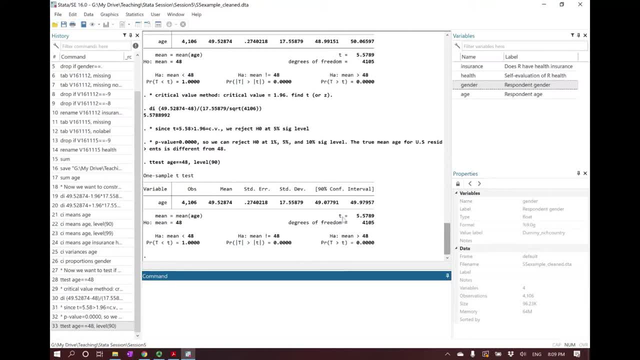 by this option at all. You see, the T statistic is still the same, The P values are still the same. The only thing that's affected is that it will override the ninety-five percent confidence interval and show a ninety percent confidence interval for you. 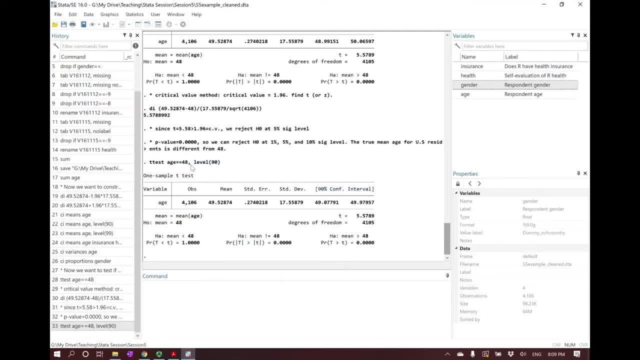 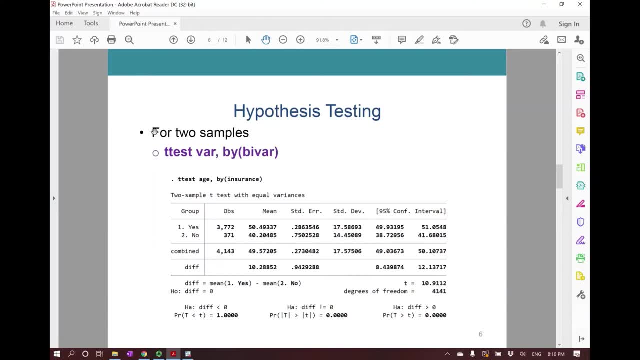 So this common, this option is always for the confidence interval. OK, So the next one. let's look at the hypothesis testing for two samples. So for two samples. usually, our research question is always to look at whether the mean is different across two different groups. 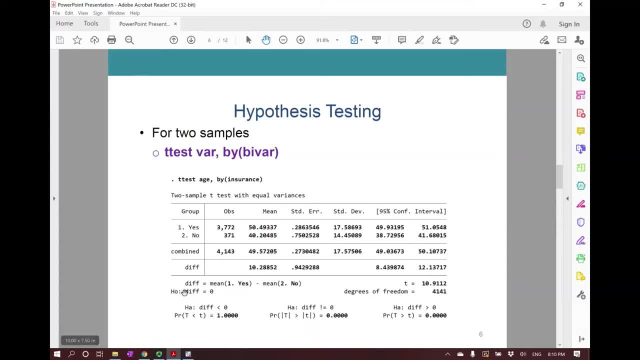 Therefore, the non-hypothesis is always that the difference is zero And, of course, the alternative hypothesis could be the case where it's not zero, it's bigger than zero or it's less than zero. So in that case, whenever we do, 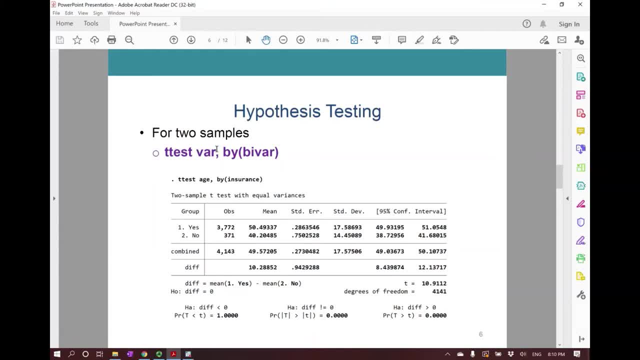 an hypothesis testing for two samples. we do not have to give and claim the value. We do not have to say: test this variable equal to something. Alternatively, we want to test this variable across some group, And I list by a: by variable. 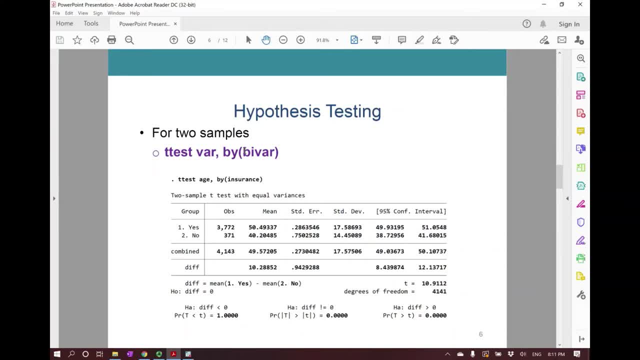 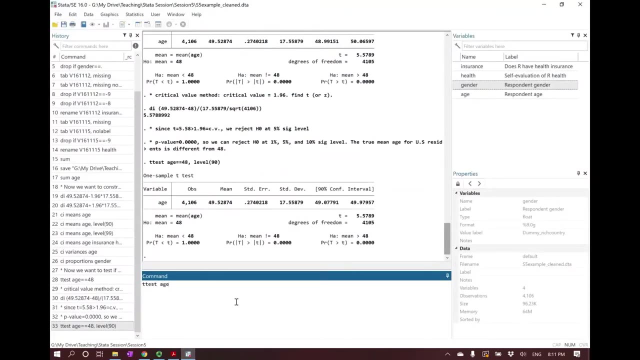 This is saying that because we are testing for two groups, we have to always have binary variables included in the parenthesis. OK, So, for example, now we would like to test the average mean, so t-test age across insurance. So we want to look at. 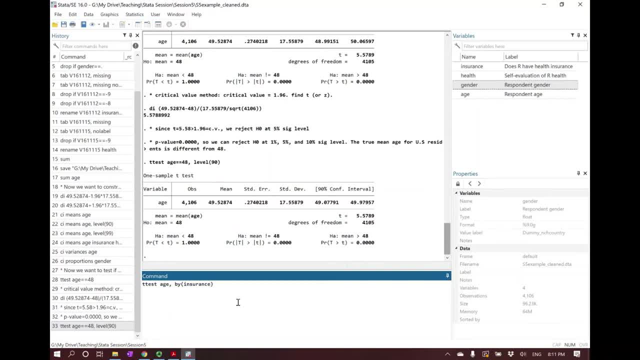 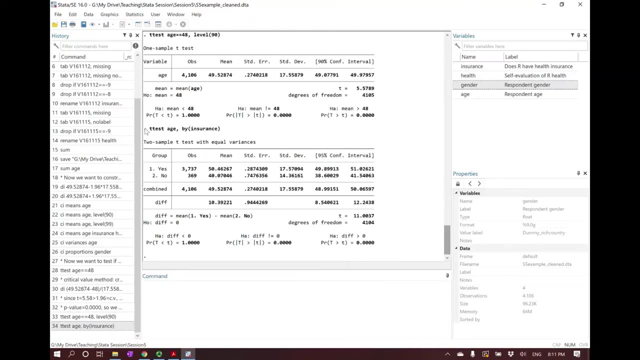 whether the mean age for US restaurants is the same as the mean age for US restaurants, whether they are different for those who have insurance and for those who does not have an insurance. OK, So if I click enter, you will see. 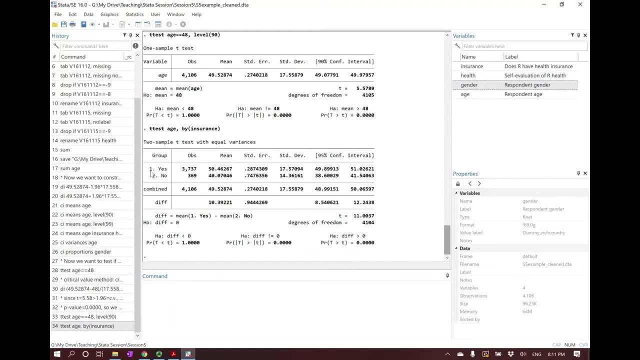 a test of results here. So first of all, it will still show you some basic descriptive statistic for all, the values for the group where insurance is one and for the other group. it will calculate the difference for you, OK. So more or less. 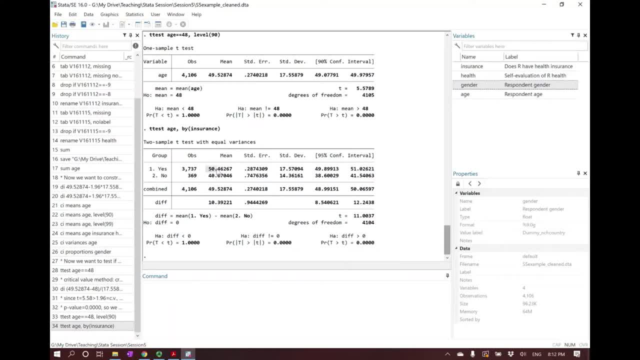 if you see that the mean age for those who have insurance is about 50 something And the mean age for those who does not have an insurance is about 40 something. So probably it's really a big difference on the mean age between the two groups. 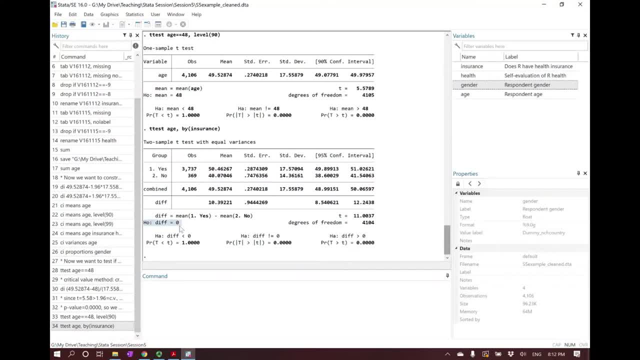 Right. So this is our non-hypothesis. and if you'd like to look at only a two-tailed test by looking at the P values here, it's pretty, pretty slow. It's just zero. This means that you can reject the non-hypothesis. 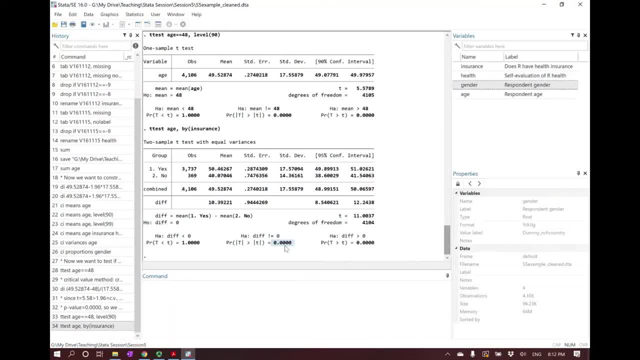 at 1 percent, 5 percent and 10 percent significant value. The mean age across those who has insurance or who does not have insurance are statistically and significantly different. OK, And at the same time, we also know that the true difference value 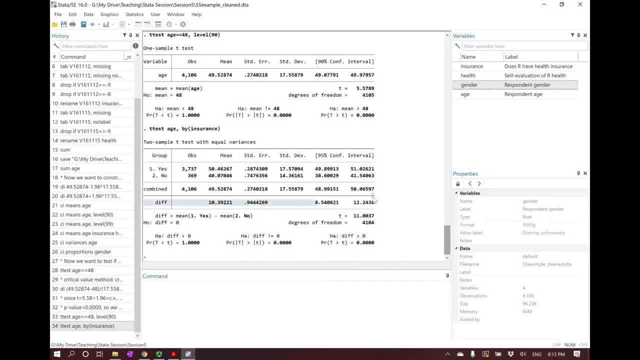 the true difference is actually from 8 to 12 something, So the true difference is a positive value. Therefore, we know that the mean age for those who has an insurance is statistically greater than those of the mean age without an insurance. OK, 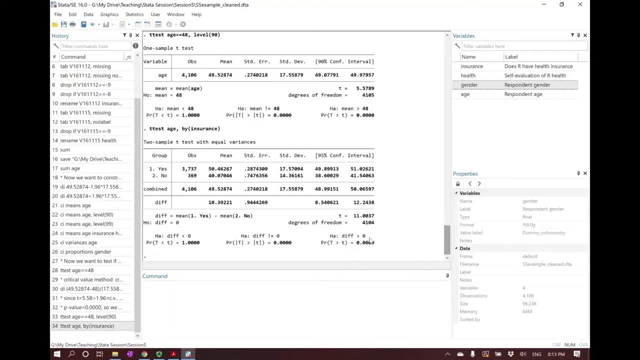 So make sure that you still intuitively understand the hypothesis test for a single sample or for two samples, Be able to still understand the critical value method or even the confidence interval method, and also be able to read the P value to quickly make rejection decision at any significant value. 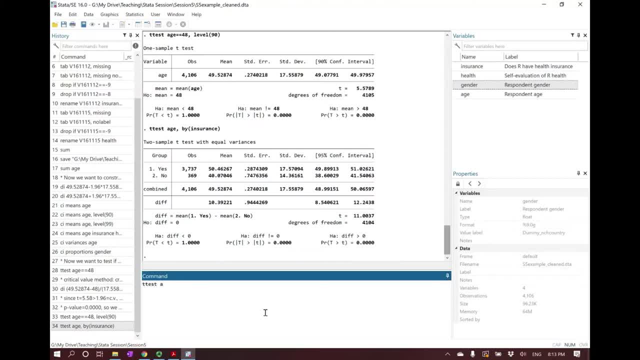 OK, So I can probably also test age across gender, So by gender. Gender is another binary variable. So if I'm testing the mean age across female and male, I can do this comment. So if I click enter and I quickly read my P values, 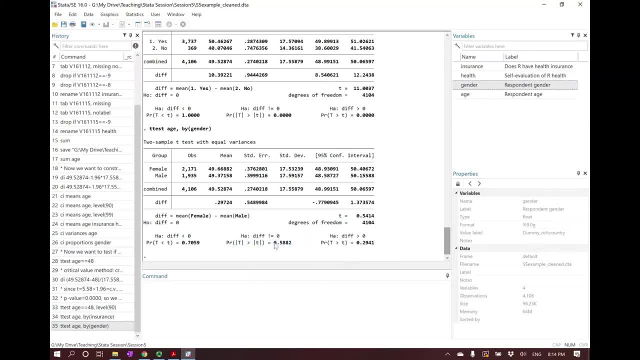 it's 0.5, 50%, So it's a very big value. Therefore I fail to reject my hypothesis at 1%, 5% and 10% significant value. So in the US there's no difference on the mean age. 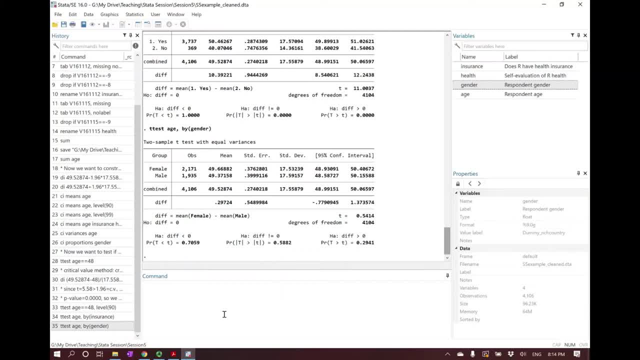 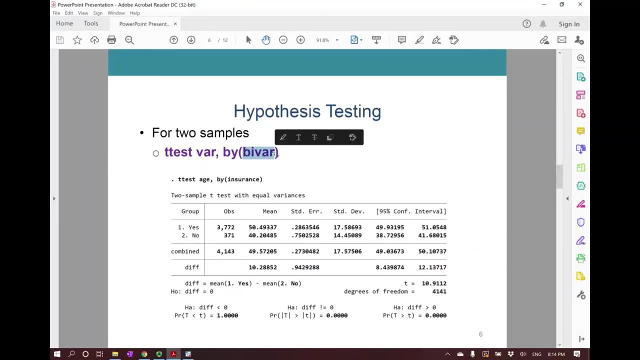 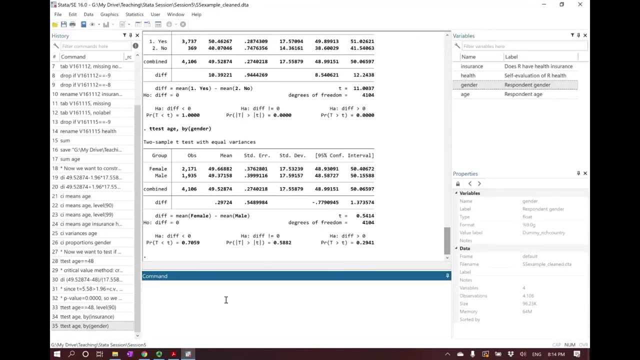 between females and males. OK, So again, it's very important to notice that we do have to have a binary variable in the parentheses. For example, we have health, which takes a value from one to five, five categories. So if you want to test, 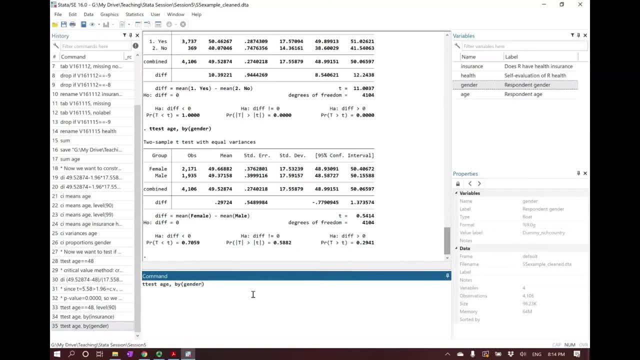 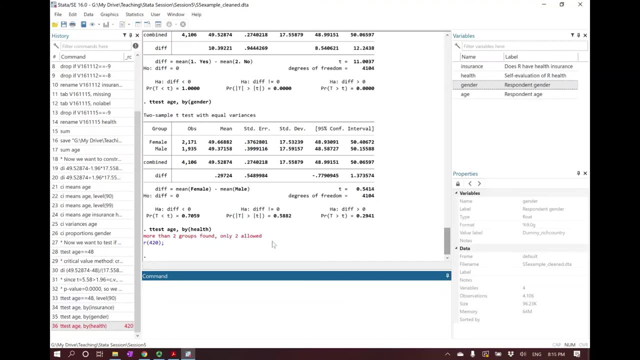 the age across different self-evaluated health status, you're going to get an error message. So, health: If you click enter, you're going to see an error message. more than two groups found only to allow Right. So if you still want to test that, 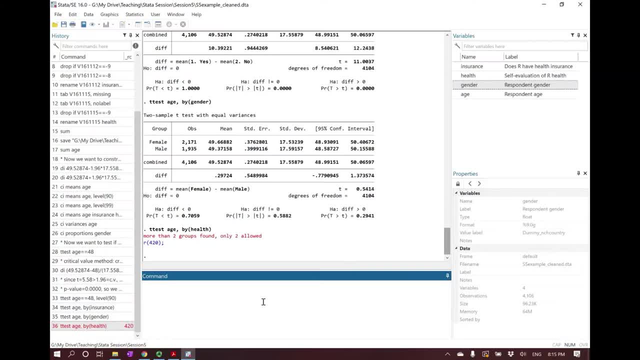 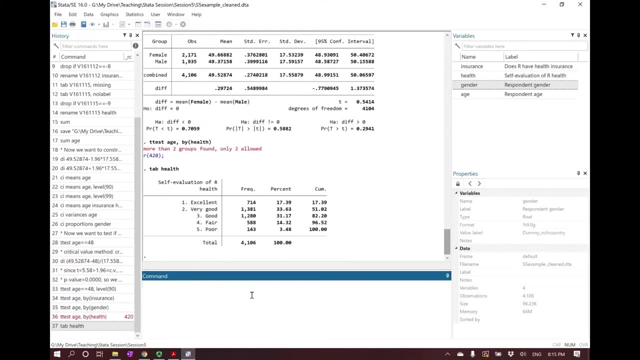 you need to find a way to regroup your health status and to create a binary variable Right. So, for example, I'm going to tab health, So I have excellent, very good, good, fair and poor, So probably I can generate. 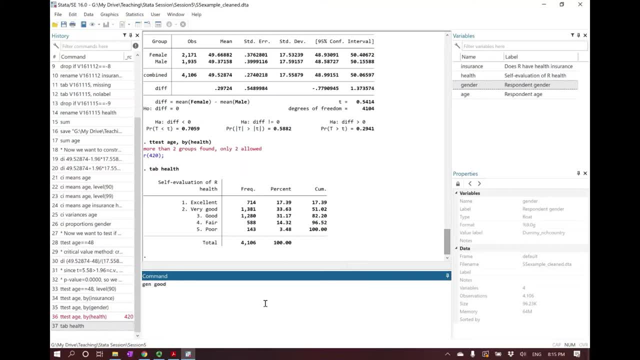 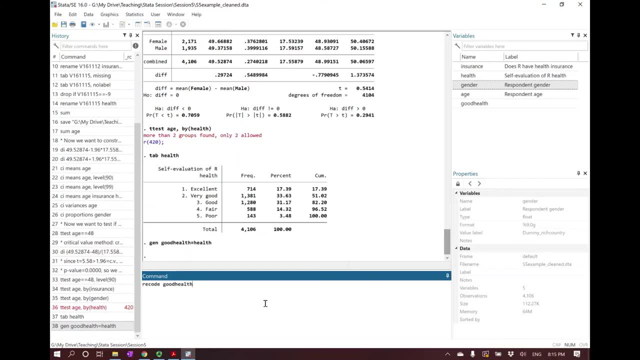 a new variable that's called good health equals to health, And I'm going to recode this good health variable so that one to three is good. So I can do from one to three being one and four, from four to five being two or being zero. 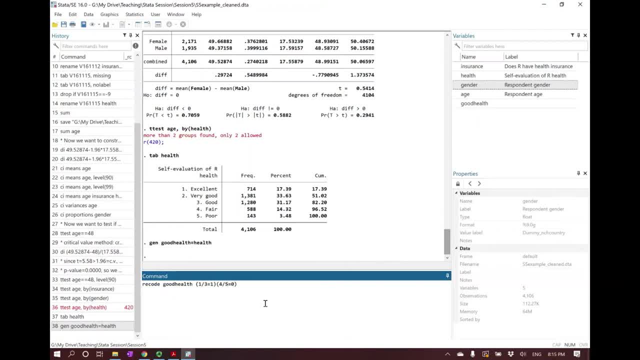 It's really up to you, as long as it's a binary variable, Right. Sometimes, if you forgot about the from and two, if it's not too many categories, you can always do one equals to one, two equals to one, three, good. 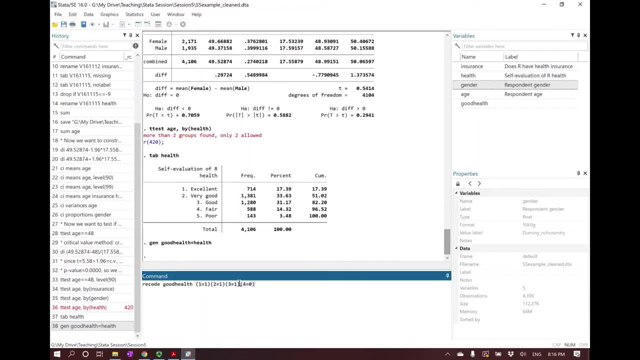 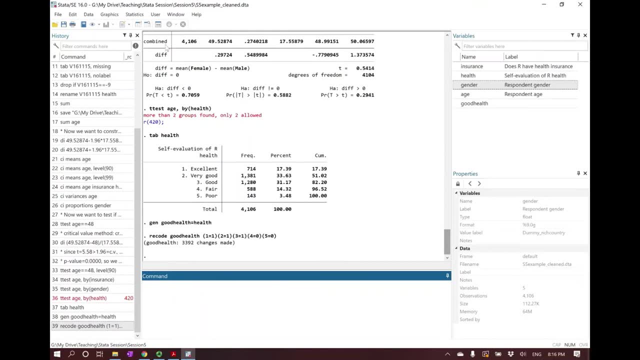 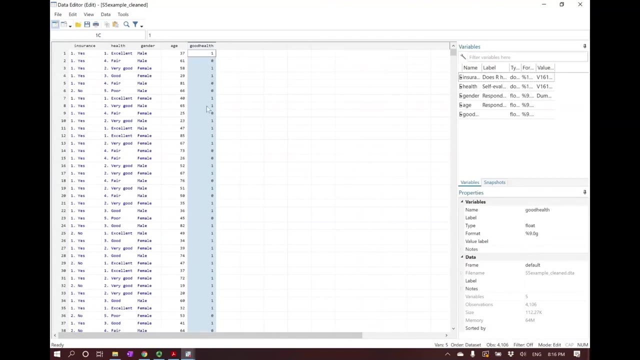 that's one, and then four being zero, five being zero, That's the same thing. Okay, So if you click enter and double check that you created a new variable that's called good health and it only takes a value of zero and one. 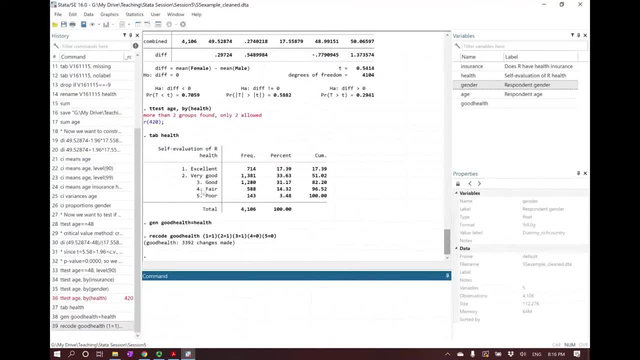 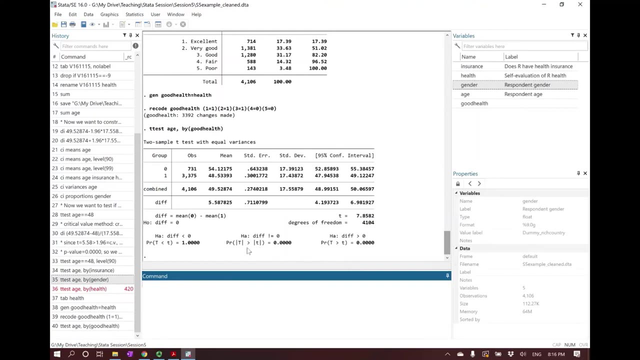 one being good health, zero being not good health, fair or poor. So now you can test the mean age across respondents with different health conditions, So by good health And if you test that hypothesis right, so the mean age for those who does not evaluate. 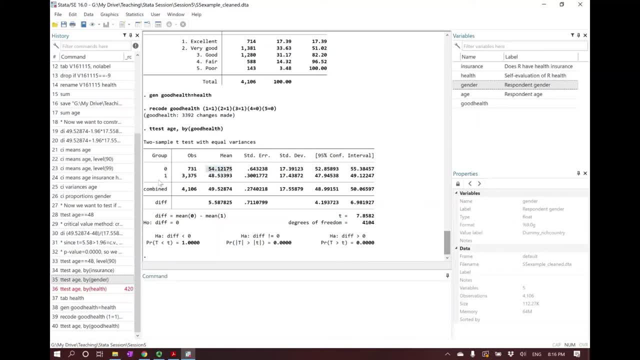 themselves with good health is around 45, and the other group is around 48. Right, So 54 and 48. So the p-value is actually zero. This means that the mean age is statistically and significantly different across the two groups: Good health and no good health. 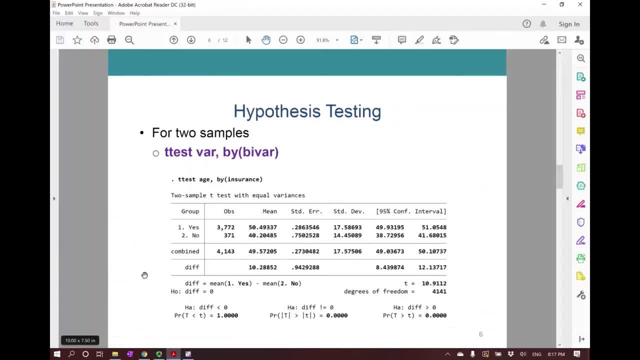 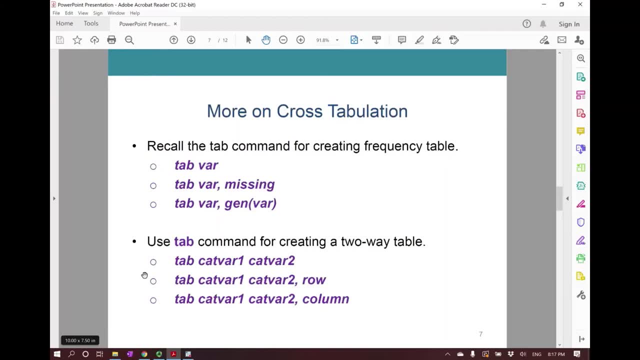 Okay, So hypothesis testing for two samples. Now I would like to talk a little bit more on the cross tabulation, also called a two-way table or a contingency table. Basically, if you recall from previously, we talked about this tab comment. 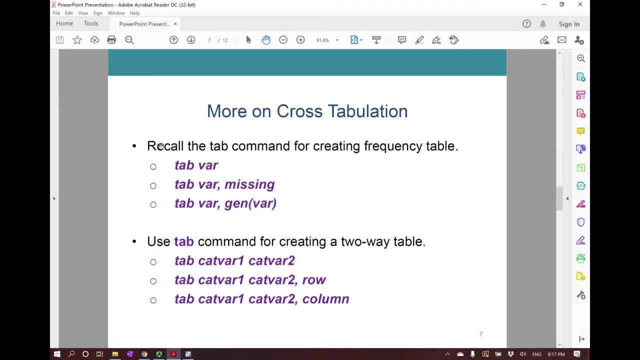 I also used this comment many times today. So if we can tab a categorical variable, we'll see some frequency tables. So a tab variable missing option. and also sometimes, if we tab the variable, we can quickly generate new binary variables for each category. 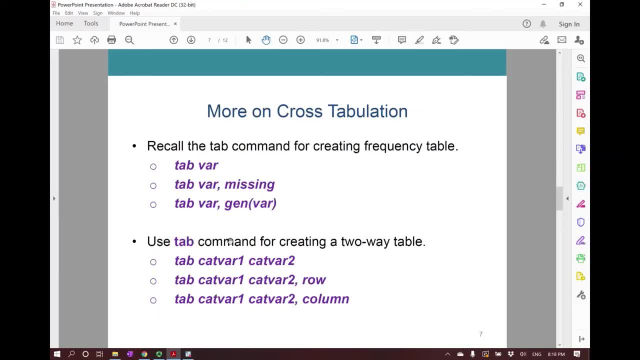 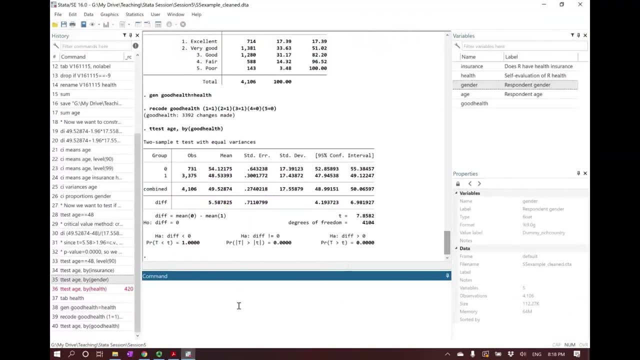 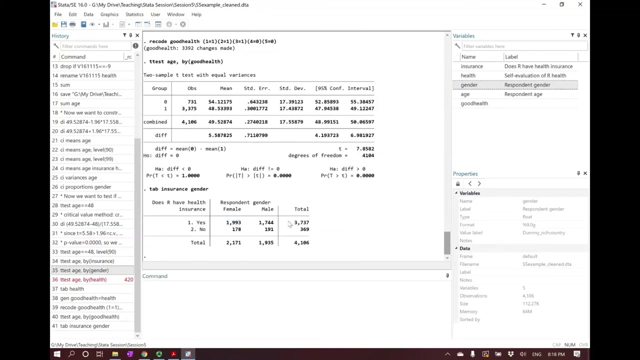 Okay, So we could also use this tab comment to create a two-way table. So basically, for example, if we tab, for example, insurance and gender, so we immediately see a two-way table and the number of observations over the total and what a proportion. 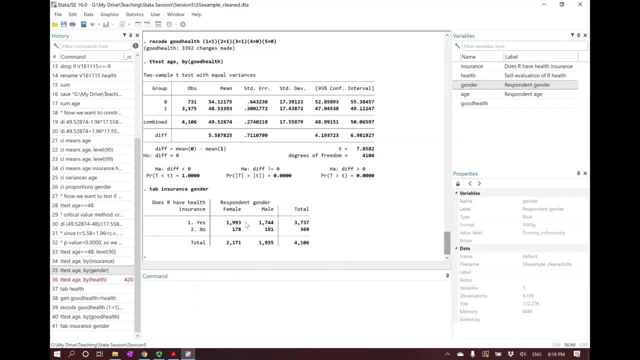 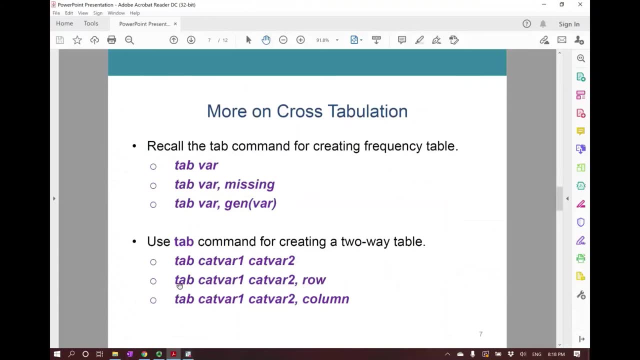 of respondents being having insurance and being female, or having insurance being male. we can easily to compare that. Okay, Actually, another option for this two-way table is you can show the percentage either crossing the row or either crossing the column. So, for example, 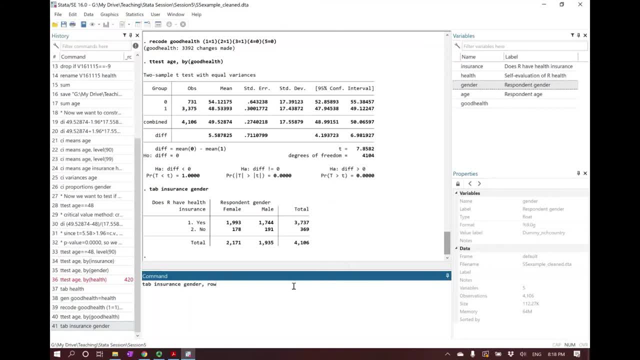 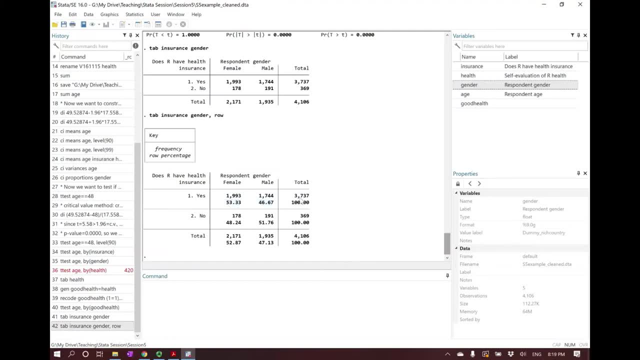 if you do tab insurance gender comma row, it will show you the percent according to the row, So the row will give you 100%. So this is to show you that among those who have insurance or who said yes for having insurance, 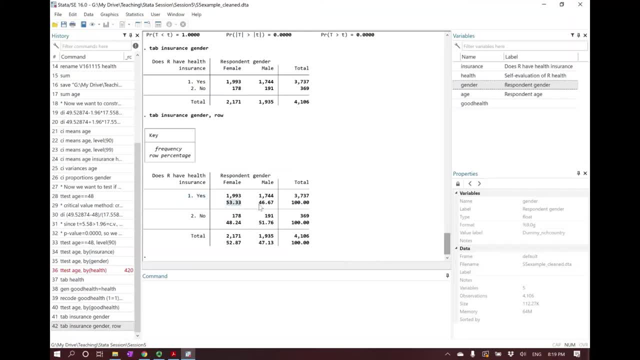 53.33% are female, 46 are male And among those who said no, 48% female and 51% male. Right: Alternatively, you can also tab insurance gender column. You can do column or just call. 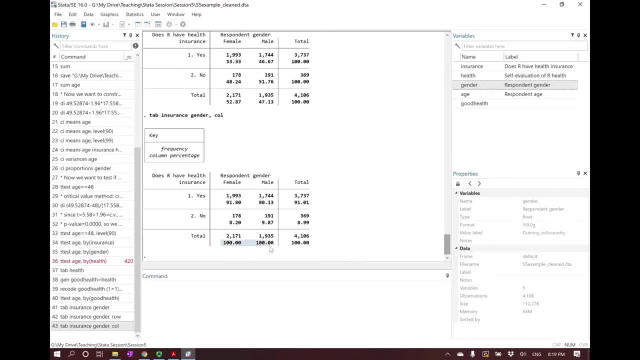 Okay, And now it will have this 100 on the columns. This is to show that, among female respondents, 91% of them have insurance and 8% does not. Among all of them, all the males, 90% have insurance. 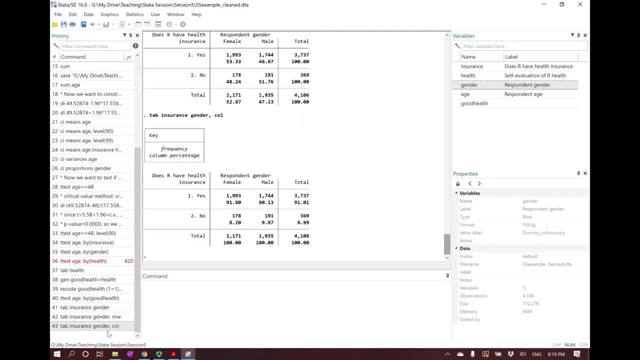 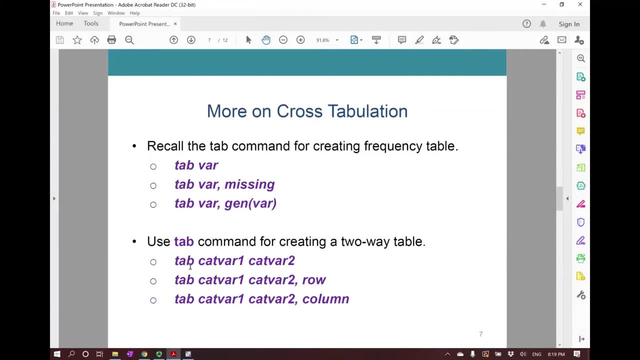 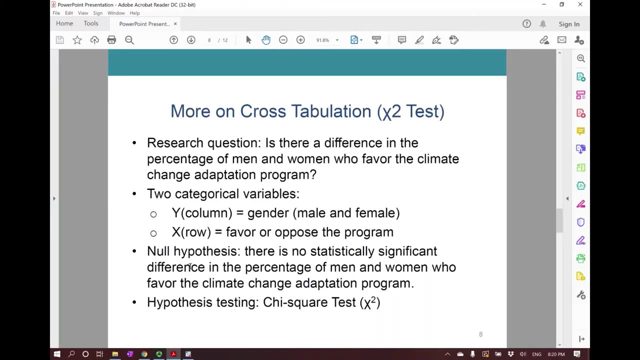 and 9% do not. Okay, These are two additional options for you, after the tab for creating a two-way table. More importantly, I'd like to introduce another type of hypothesis testing, which was not covered in the regular lecture, So sometimes. 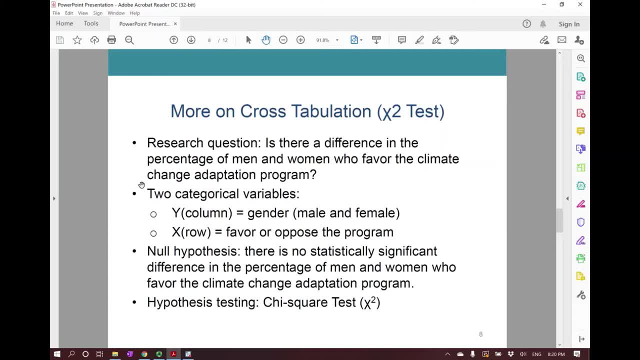 we do want to do some categorical data and then do some data analysis. Instead of asking if there's any differences in the mean age of quantitative data across different groups, sometimes we may just want to know the difference between two groups across other groups. 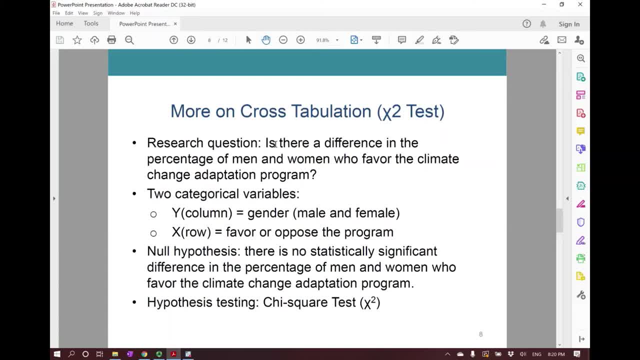 Right. So, for example, a research question could be: I want to know if there's any difference between male and female or in the percentage of male and female who favor the climate change adaptation program. So I would actually be examining two categorical variables. 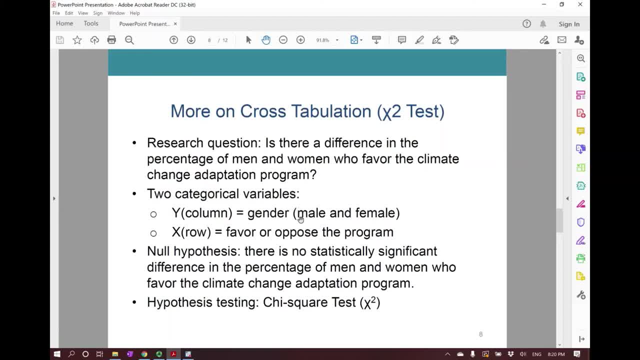 One is the gender, which is male and female, zero, or one Another one is going to be my role variable, that is a favor or oppose. Okay, So then our non-hypothesis is to say that there's no statistically significant difference in the percentage. 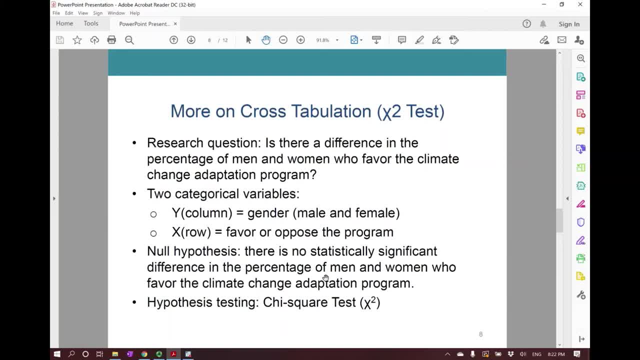 of men and women who favor the climate change adaptation program, And the hypothesis testing that we're going to do is called a chi-square test. The symbol is called a chi chi-square. Okay, Although this is a different type of hypothesis testing. 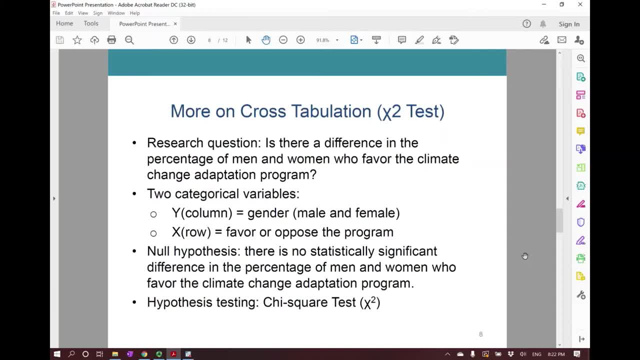 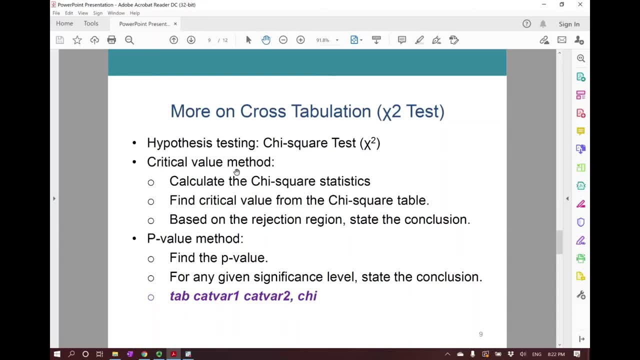 but the key steps or the methods for hypothesis testing are exactly the same. You could do a critical value method, which is to calculate a chi-square statistic. Okay, And then we're going to examine categorical variables. Therefore, those variables will not have a normal 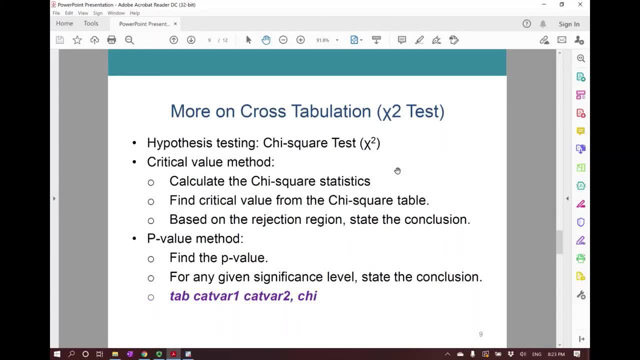 distribution. Instead they have a chi-square distribution, which I will not talk in depth, But because it has a chi-square distribution, we're going to calculate a tested statistic that is called a chi-square statistic, Okay, And then we can look at. 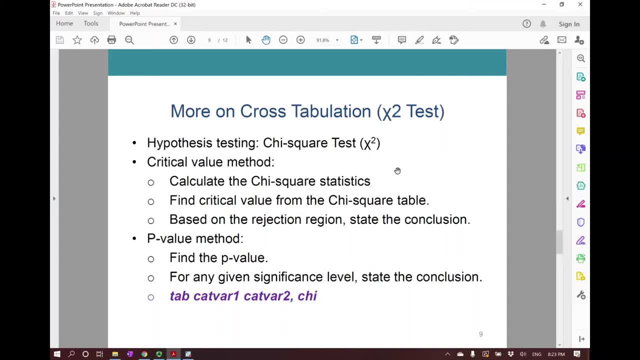 the statistic and the critical value. then we can look at the rejection decision, look at the rejection region and state the conclusion. So exactly same idea for any hypothesis testing. Alternatively, and also very commonly used in empirical research, is: we'll look at a chi-square test. 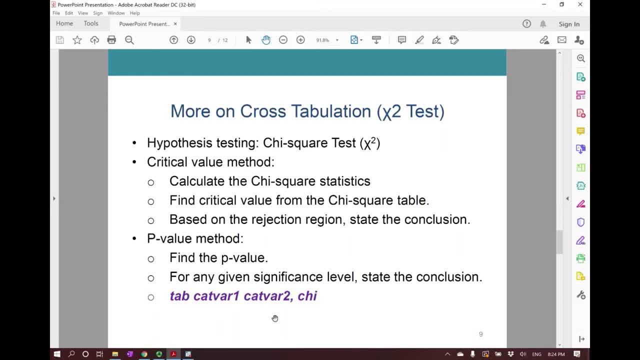 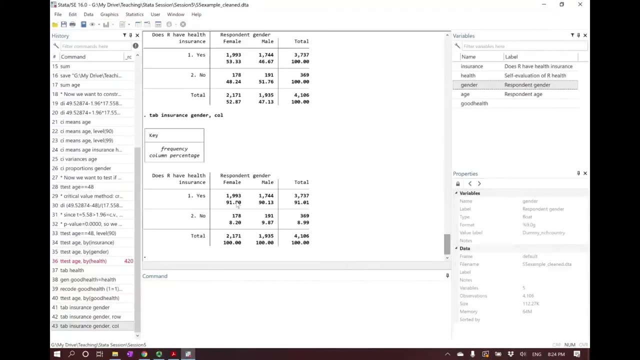 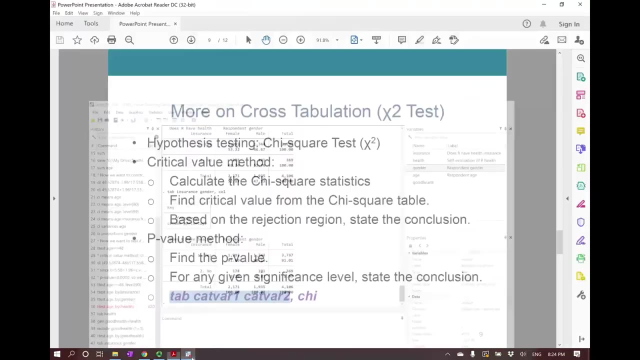 and then, for any given significance level, we can state our conclusion. Okay, So the state of comment for chi-square test is: you're still going to tap the two categorical variables you are interested to, But other than just test at the same time, which just? 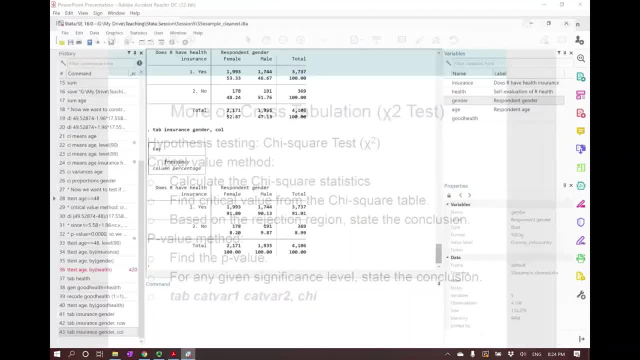 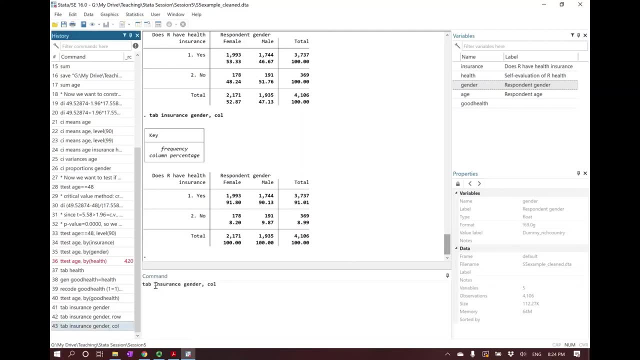 to additionally give comma c-h-i. So, for example, right now I'm going to do- I want to look at, for example, female and male who are, whether there's a gender difference in terms of purchasing insurance. So, probably one on the row, one on the. 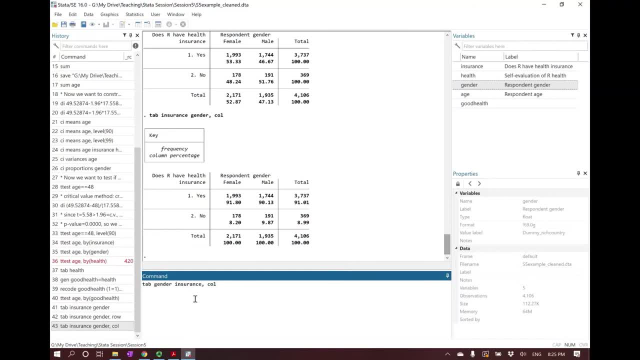 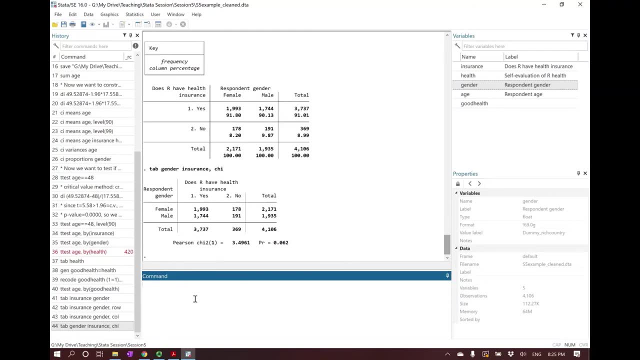 column and one on the row, So the option is going to be c-h-i. Okay, So if I click enter, I'm first. I'm still going to see this frequency table, or two way table. Alternatively, Stata will. in this case, we have 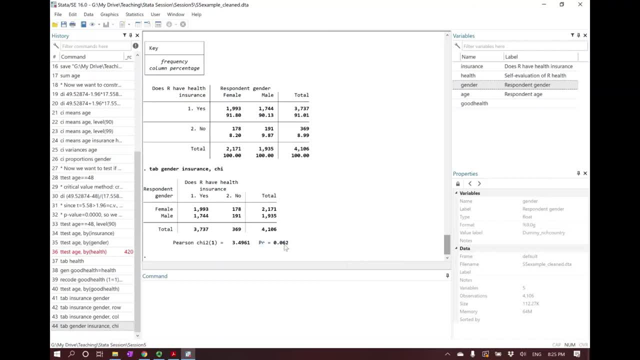 a p-value which is point zero, six. Okay, So it's six percent. This is to say that we can reject the non hypothesis at ten percent, but we cannot reject the non hypothesis at one percent or five percent. Right, Remember? how do we? 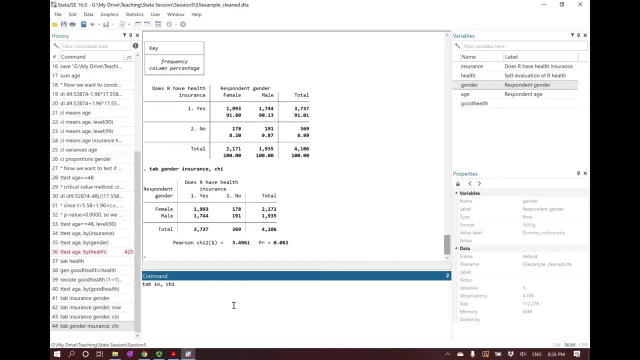 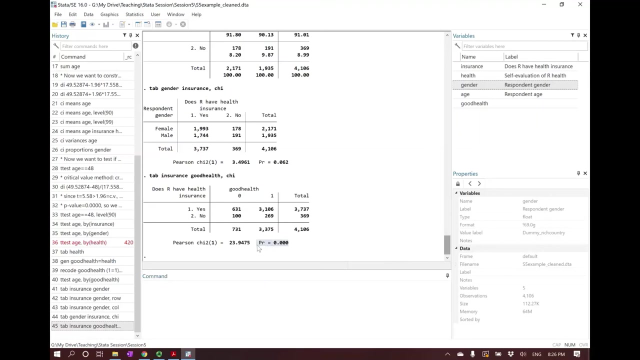 look at insurance and health. So let's first look at insurance and good health. So we want to look at whether the percentage of respondents purchasing or not purchasing insurance- if it makes a difference for having a good health. I have a very big p-value. 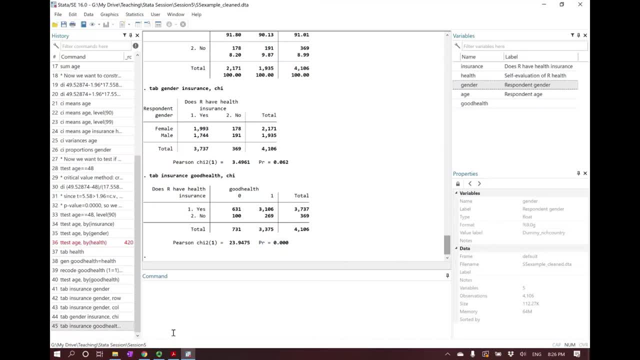 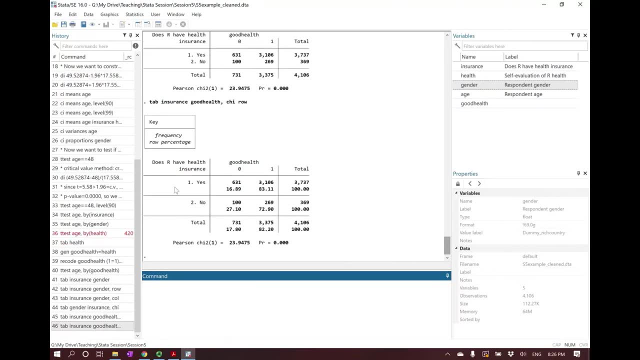 as expected, Right? So actually, for those who do, you can still do the option, for example, roll. So for those who purchased the insurance, eighty percent of them self-evaluated to have a good health, And for those who does not have good health,